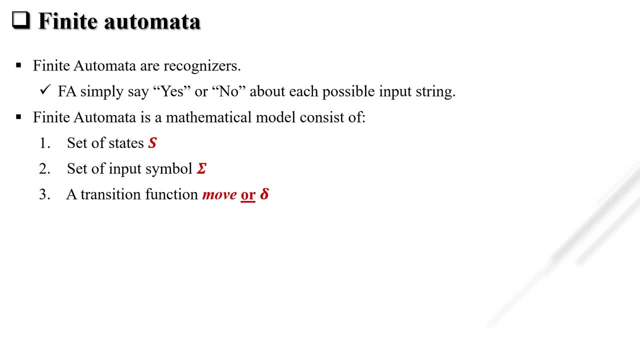 or move function. it is also known as transition function. fourth, s0, or you can also use I- 0. it is an initial state of any NFA or DFA for any finite rotameter, and the fifth one is F- it is an accepting state or final state. 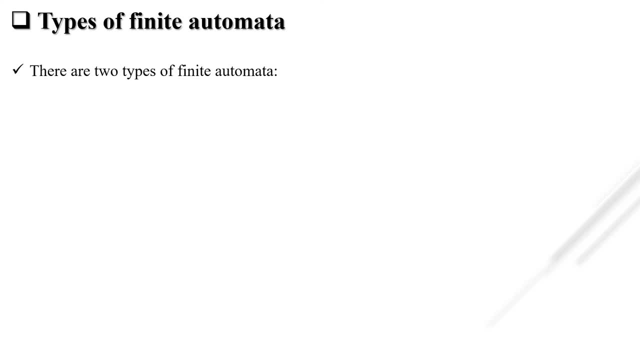 so there are two types of finite rotameter. first one is DFA, that is, deterministic finite rotameter, where for each state exactly one edges living out for each symbol. let understand with this example: here you see that from each state only one edge is living out for a or B. in DFA, from one state, two edges of same symbol. 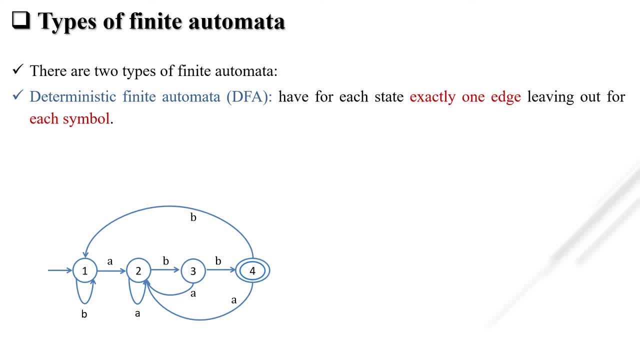 is not permitted, okay. so, as you see here, suppose from 1 to 2, there is a edge of a living out to 2. so what is not permitted? from 1? it is not permitted to take a same symbol to another state. okay, it is wrong. similarly, from 3, only one B symbol is reaching to 4. 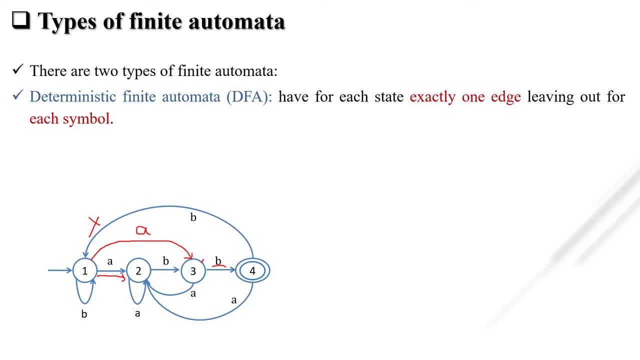 okay, there is no other B symbol reaching a living out from 3. okay, the next one is NFA, that is, non-deterministic, finite restiction子. also, some ages are labeled with the null symbol. let's understand with example. so here you see that the symbol a from initial state reaching to initial state, as well as 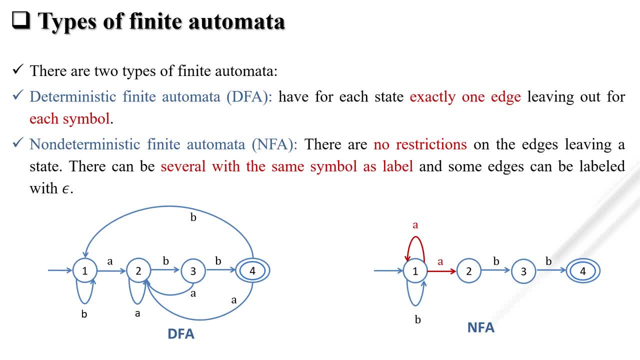 to the other state that is from 1 to 2 and from 1 to 1 also. okay in an NFA. it is also possible that here there is a age B is living from 2 to 3. it may be possible it is living from 2 to 4, so same. 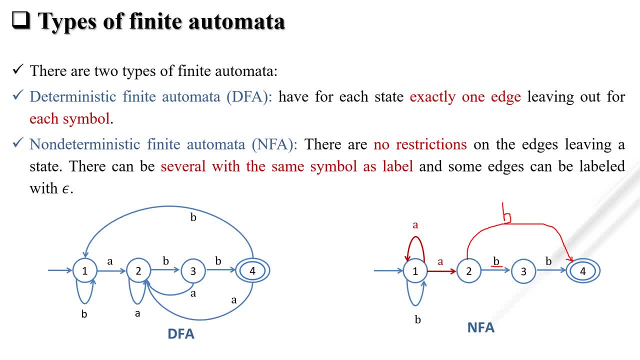 symbol can be reached from 2 to 4 and 2 to 3. okay, it is permitted in NFA, but it is not permitted in DFA. so in DFA, exactly one edges of same symbol is living out, but in NFA there is no restriction on the edges living a state with the same symbol. okay, 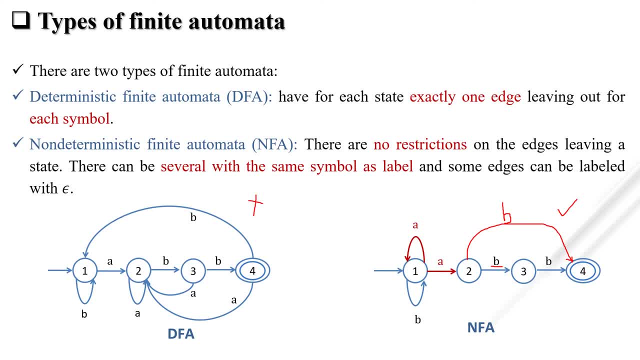 now clearly you can see here 2 to 3. suppose in DFA 2 to 3, B symbol is leaving. okay from 2 to 3, but 2 to 4 or 2 to any other state it is not happening. okay in DFA, but in NFA it is possible. 1 to 1 is. 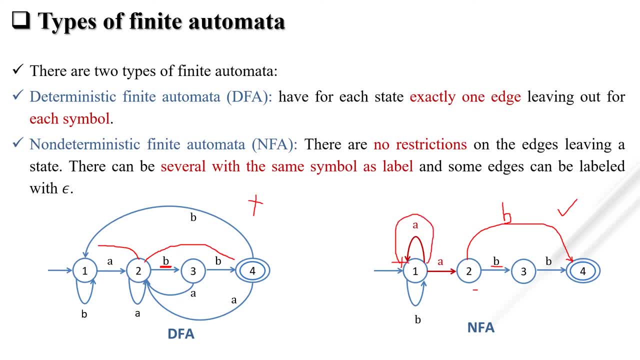 also happening. A transition, okay. and in DFA it is possible. 1 to 1 is also happening. okay, and in DFA it is also possible. 1 to 1 is also happening. A transition, okay. and in NFA it is also possible. one to 2 is also happening. so the multiple symbol in NFA is allowed. 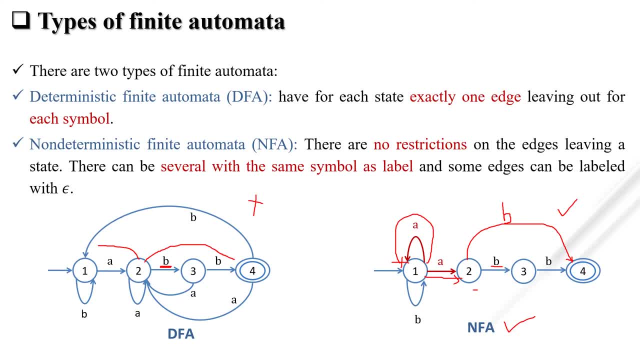 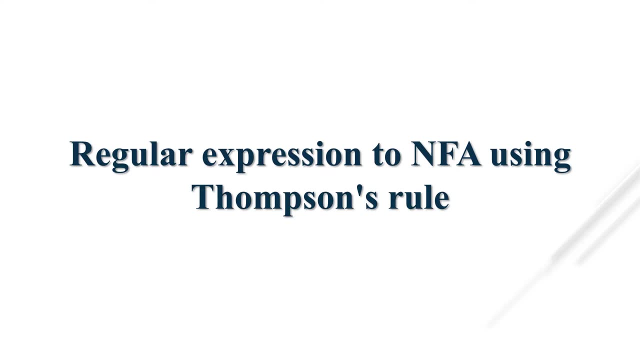 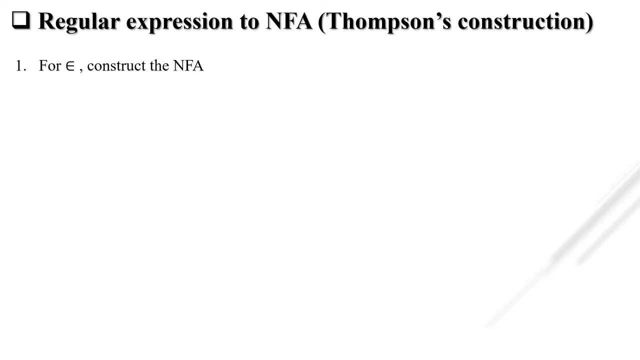 we can go from one state to the other state with the same symbol, but in DFA it is not permitted. okay, now we see how NFA is constructed from Re, using Thomson rule. so for null, the NFA is of two state. first is initial state that is represented as I here, and second is 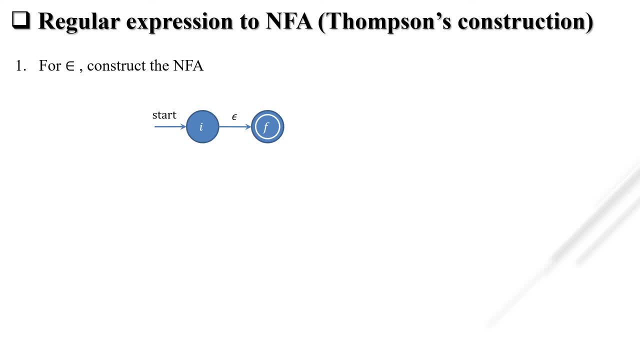 final state, which is represented as F here and it, the final state is also represented as double circle. also, the initial state is defined as this arrow. this is compulsory to put at the start symbol, okay, otherwise your NFA is going to wrong. so similarly for the symbol. a NFA is of two state. first one is: 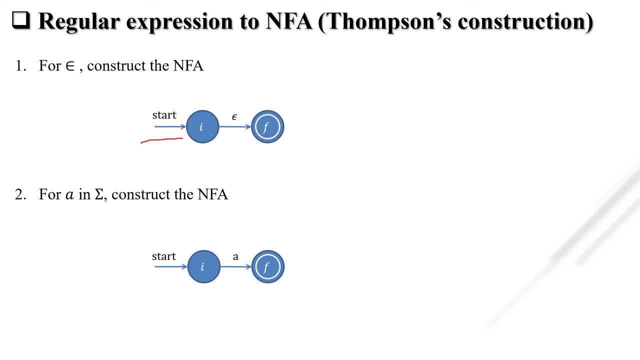 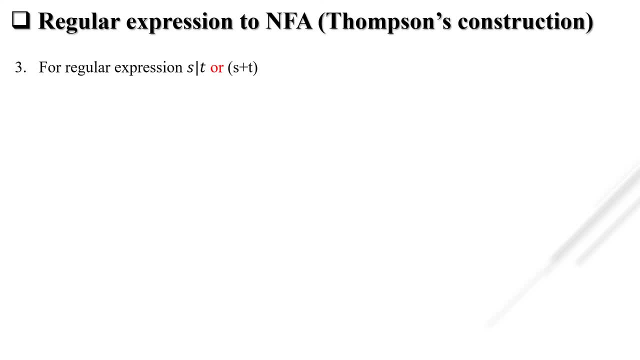 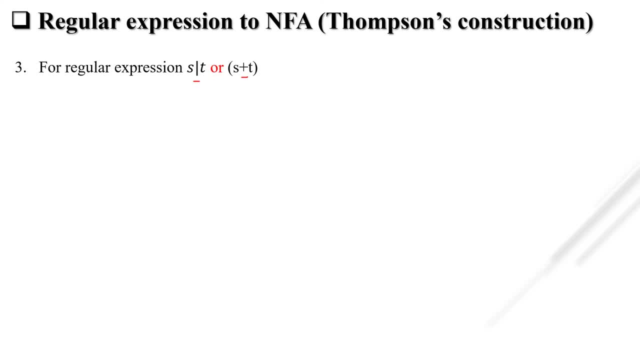 for this plus notation. okay, it is a for this plus notation. okay, it is a symbol for R, as we already see in symbol for R, as we already see in symbol for R, as we already see in regular expression. so for this re there, regular expression. so for this re there. 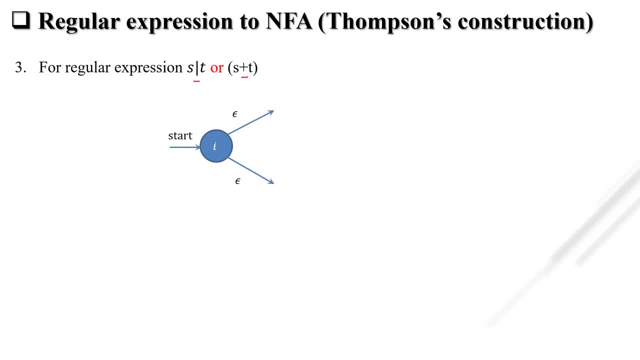 regular expression. so for this re there is a transition of null from initial. is a transition of null from initial. is a transition of null from initial. state of n of s and n of okay. also there. state of n of s and n of okay. also there. state of n of s and n of okay. also there is a transition. 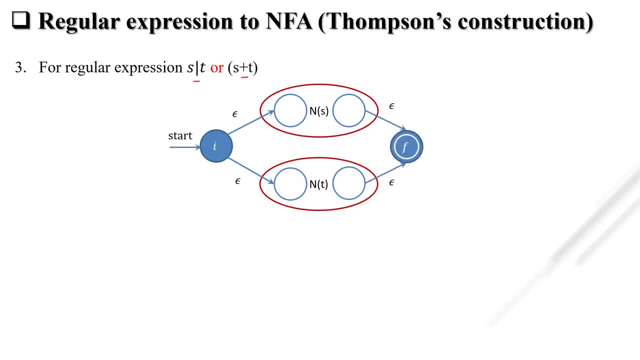 is a transition is a transition on null to the final state of n of s and on null to the final state of n of s and on null to the final state of n of s and n of t. so this is a Thompson rule for n of t. so this is a Thompson rule for. 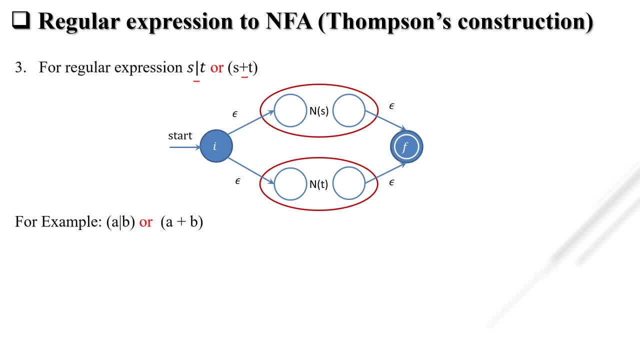 n of t. so this is a Thompson rule for our notation. let's see the example here, our notation. let's see the example here, our notation. let's see the example here: we construct an FFR a or B, so the NFA. we construct an FFR a or B, so the NFA. 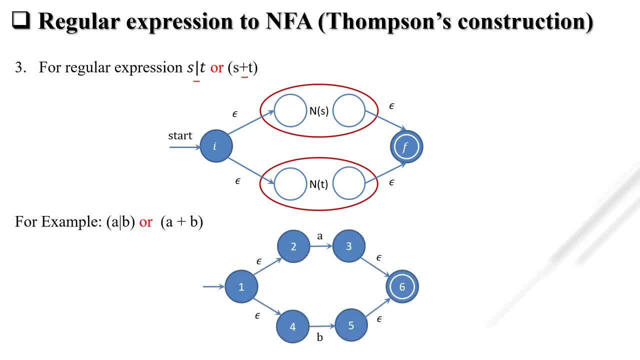 we construct an FFR a or B, so the NFA is here also there is a transition on is here also there is a transition on is. here also there is a transition on null, from one that is our start state to null, from one that is our start state to. 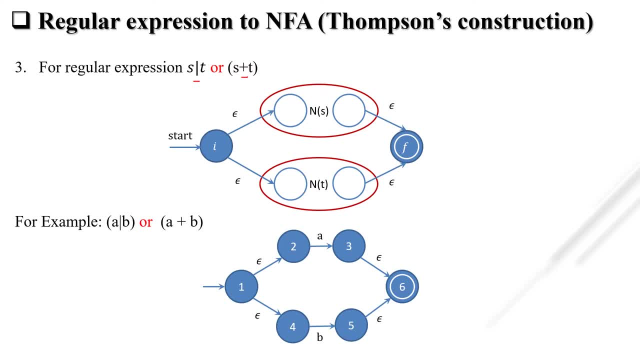 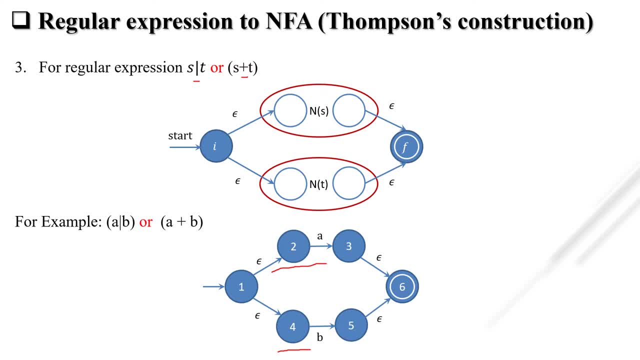 and this B also. there is a transition, and this B also. there is a transition on null, from the accepting state of a from on null, from the accepting state of a from on null, from the accepting state of a, from the accepting state of a and B to the. 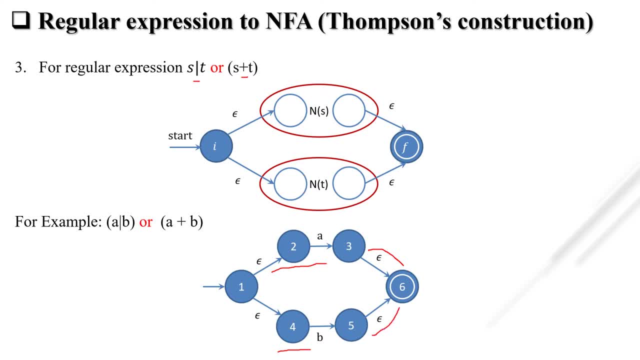 the accepting state of a and B to the. the accepting state of a and B to the new accept accepting state: that is 6- okay. new accept accepting state: that is 6- okay. new accept accepting state: that is 6- okay. so the BB or operator. so the BB or operator. 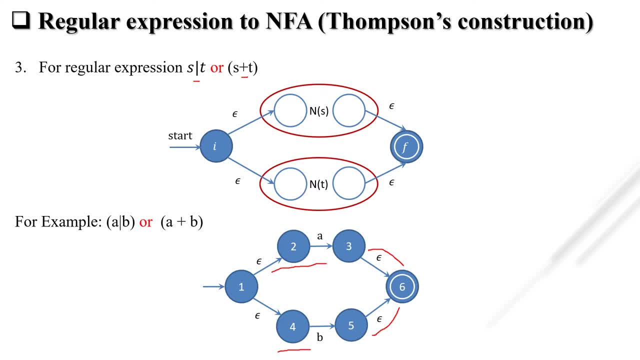 so the BB or operator will be in re. so we have to do two parts first. will be in re. so we have to do two parts first. will be in re. so we have to do two parts first, like we have done a part first and like we have done a part first and 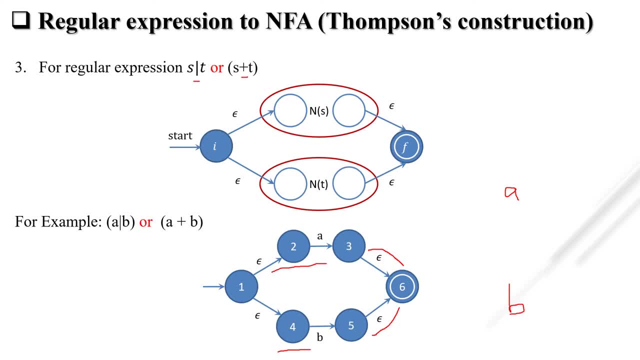 like we have done a part first and become, become, become okay with, okay with, okay with the directed draft from one state to the directed draft from one state to the directed draft from one state to another state. this is also a directed another state, this is also a directed. 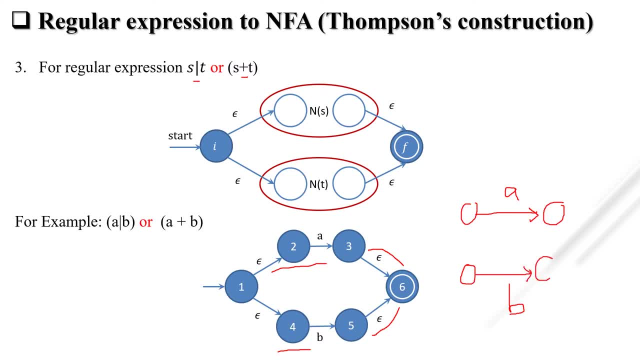 another state. this is also a directed draft from one state to another state, draft from one state to another state, draft from one state to another state. then what we have to do is simply a. then what we have to do is simply a. then what we have to do is simply a state as an initial state ahead, and 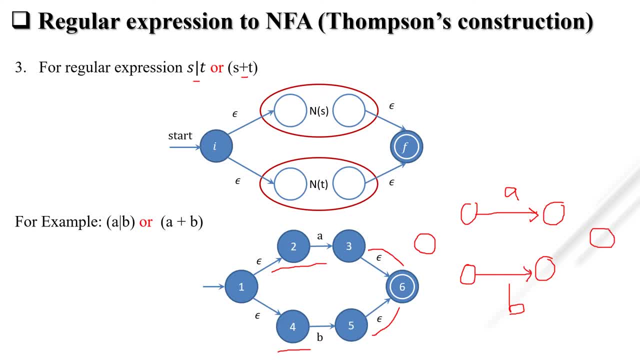 state as an initial state ahead and state as an initial state ahead and at the last, and this is also directed at the last, and this is also directed at the last, and this is also directed with null. yeah, yeah, similarly from here, with null. yeah, yeah, similarly from here. 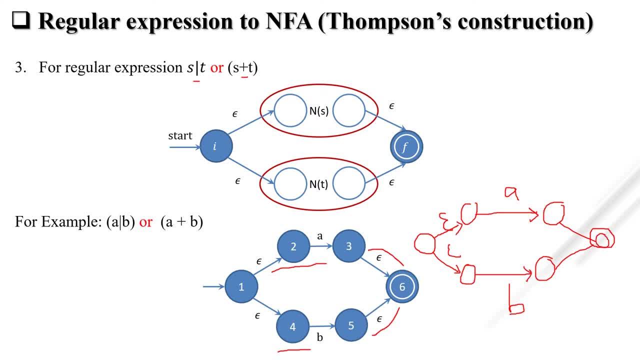 with null. yeah, yeah, similarly from here. yeah, this is our final state for a or B. yeah, this is our final state for a or B. yeah, this is our final state for a or B. and what is our first initial state? this? and what is our first initial state? this? 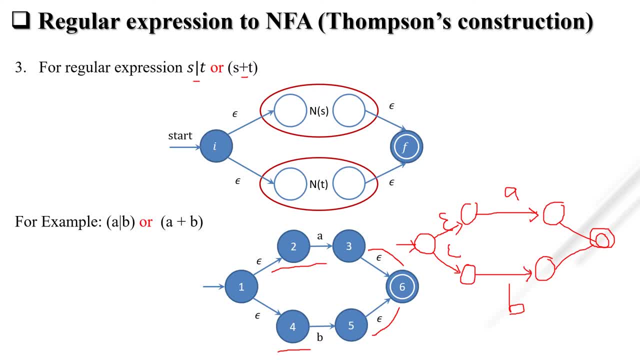 and what is our first initial state? this one. so you have to represent it with one. so you have to represent it with one. so you have to represent it with this arrow. okay, the yeah pap is the this arrow. okay, the yeah pap is the this arrow. okay, the yeah pap is the state's course. zero, say, be numbering. 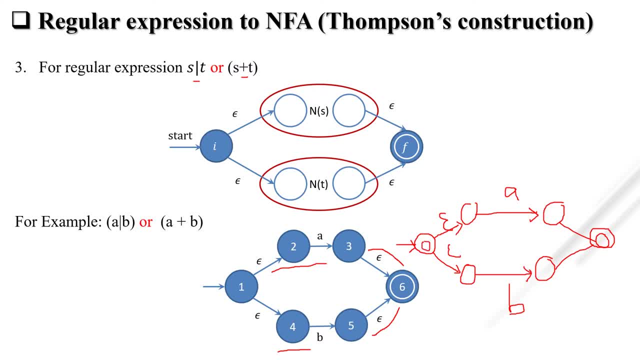 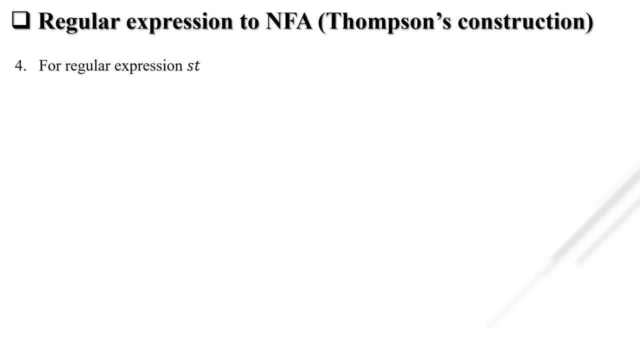 state's course zero say: be numbering. state's course zero say: be numbering they sector once every. that's they. they sector once every. that's they. they sector once every. that's they sector or issue name. okay, so the next is construct an NFA for the. so the next is construct an NFA for the. 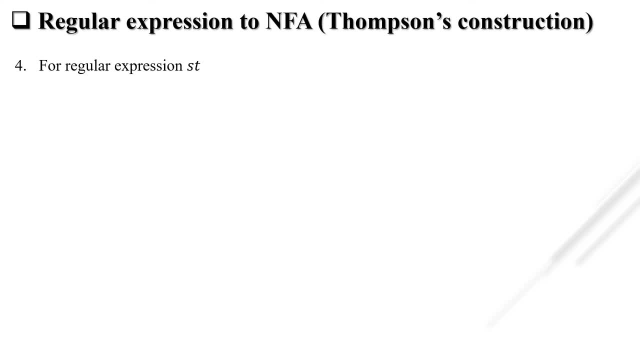 so the next is construct an NFA for the regular expression ST s is concrete regular expression. ST s is concrete regular expression. ST s is concrete, concatenate with T. so there is a start concatenate with T. so there is a start concatenate with T. so there is a start symbol. it is initial state I and there 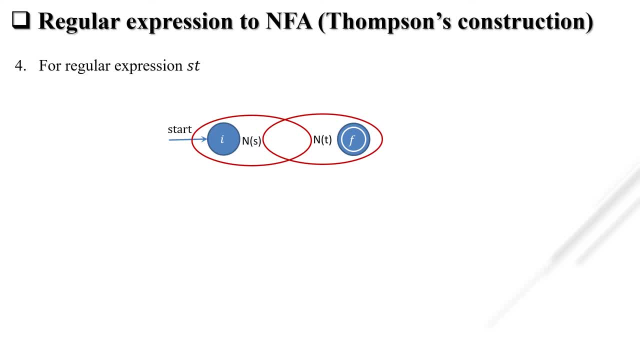 symbol: it is initial state I and there symbol: it is initial state I and there is a final state and both are concrete. in is a final state and both are concrete in is a final state and both are concrete in it. let's see with example, for example: 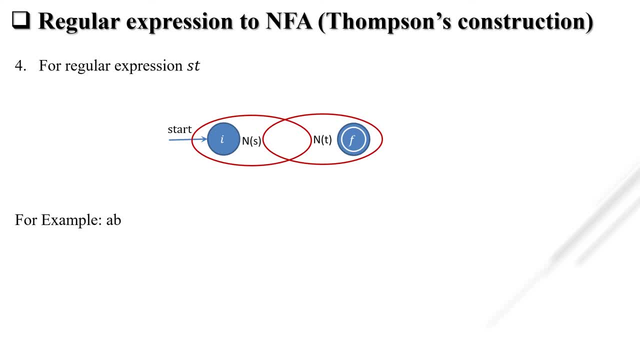 it. let's see with example, for example, it. let's see with example, for example: the R is a- B. this concatenate with each, the R is a- B. this concatenate with each. the R is a- B. this concatenate with each other. then the NFA is a and B. here. 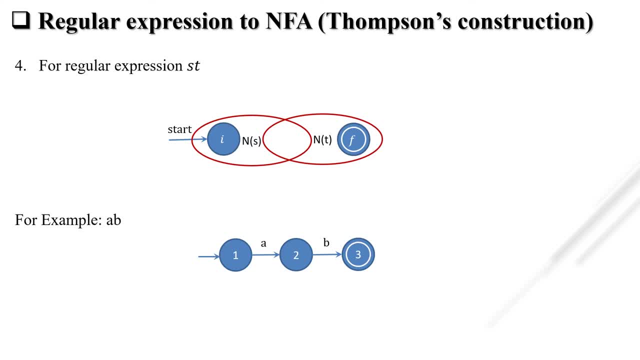 other than the NFA is a and B here. other than the NFA is a and B here, there is no null. if there is a, there is no null. if there is a, there is no null. if there is a concatenation, there is no null. okay, so. 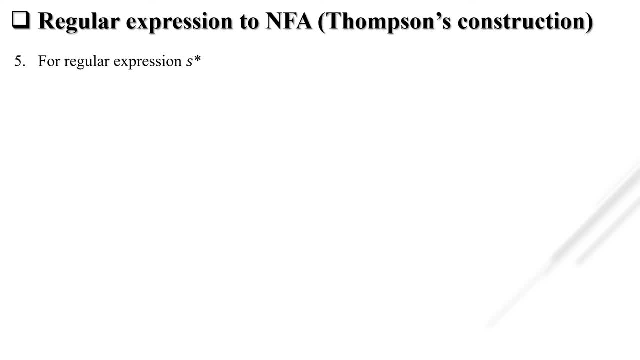 concatenation: there is no null, okay. so concatenation: there is no null, okay. so the next one is draw the NFA for s. the next one is draw the NFA for s. the next one is draw the NFA for s star: here it is a clean closer. so for 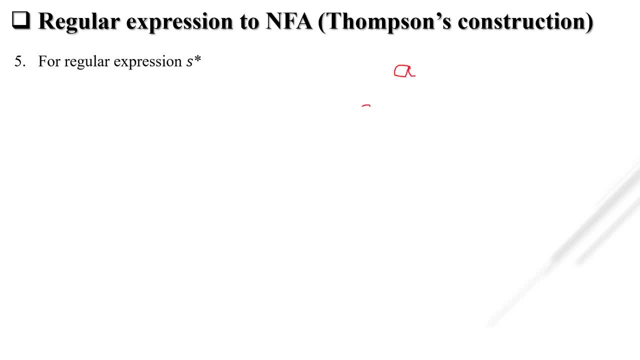 star: here it is a clean closer. so for star: here it is a clean closer. so for simple a. what is our NFA? simple a. what is our NFA? simple a. what is our NFA? simply one initial state and one final. simply one initial state and one final. 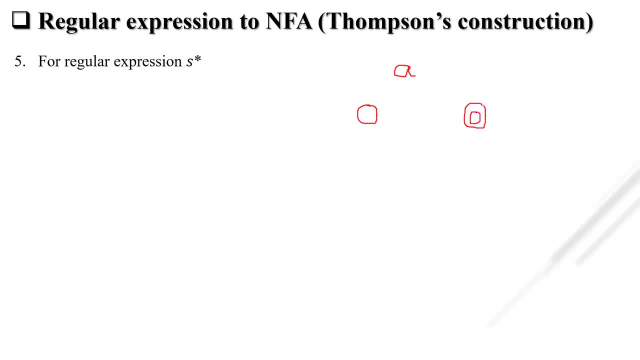 simply one initial state and one final state. okay, and H is living from initial state. okay, and H is living from initial state. okay, and H is living from initial state to final state with the symbol a. state to final state with the symbol a state to final state with the symbol a. okay, this is a start state, this is a. 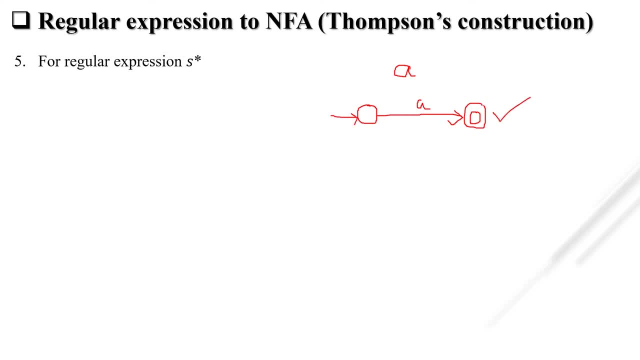 okay, this is a start state. this is a. okay, this is a start state. this is a NFA for only symbol a. so what what if NFA for only symbol a? so what, what if NFA for only symbol a? so what, what if there is a clean closer? that is a star. 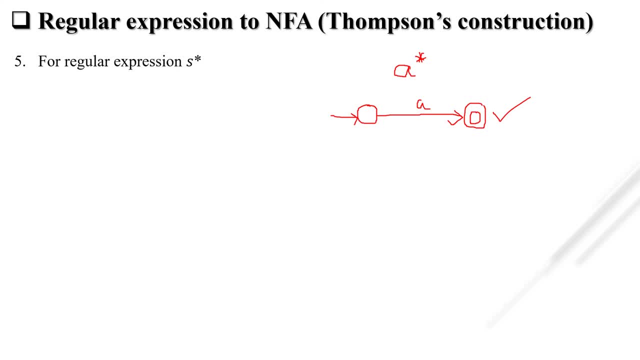 there is a clean closer, that is a star. there is a clean closer, that is a star, then how to draw NFA using Thompson rule. then how to draw NFA using Thompson rule. then how to draw NFA using Thompson rule: same, we have one. same we have one. 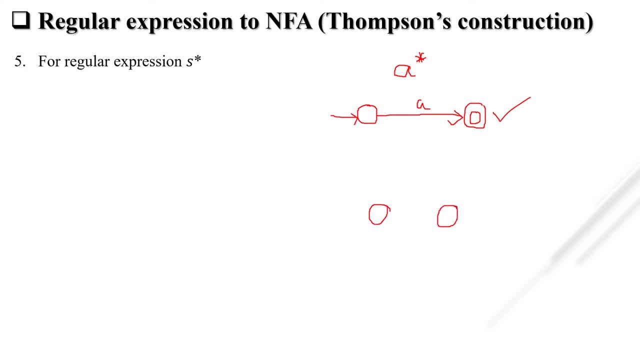 same. we have one initial state, one final state which is initial state, one final state which is initial state, one final state which is leaving an edge with the symbol a okay. leaving an edge with the symbol a okay. leaving an edge with the symbol a okay. so we have to insert one state at the 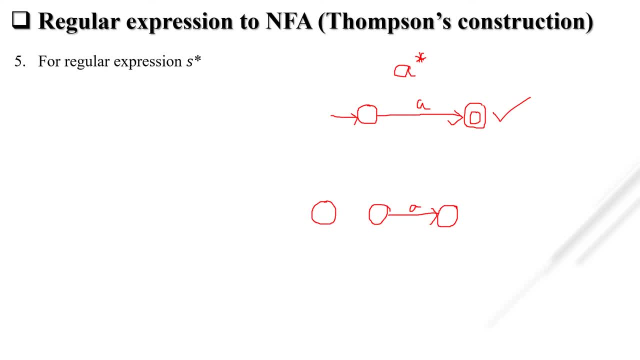 so we have to insert one state at the. so we have to insert one state at the beginning and one state at the end of beginning and one state at the end of beginning and one state at the end of the end of the NFA. okay, with the edges. 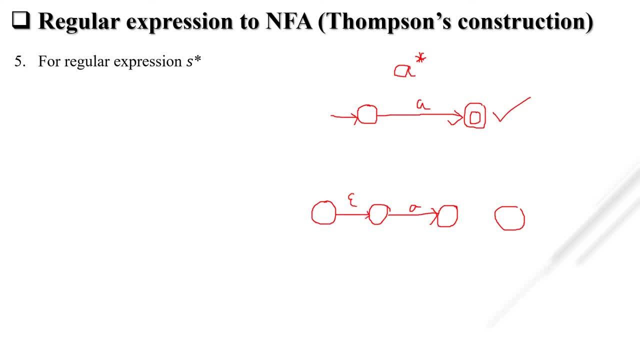 the end of the NFA. okay with the edges. the end of the NFA, okay with the edges. null here also near us. null here also near us. null here also near us. okay, this is our final state and this is okay. this is our final state and this is. 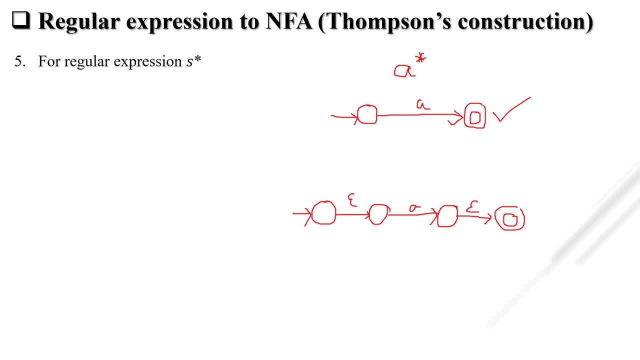 okay, this is our final state and this is a initial state according to Thompson, a initial state according to Thompson, a initial state according to Thompson rule. we have to put an directed graph rule. we have to put an directed graph rule. we have to put an directed graph from n state of a to the starting state. 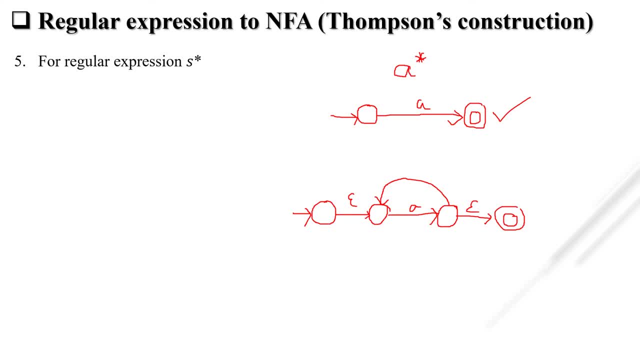 from n state of a to the starting state. from n state of a to the starting state of a and the original initial state to of a and the original initial state to of a and the original initial state to final state. there is one directed arrow. final state. there is one directed arrow. 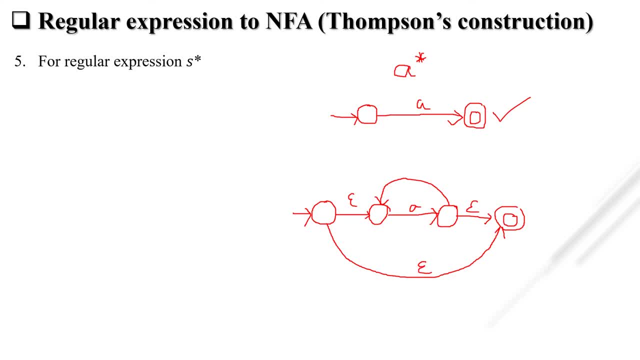 final state. there is one directed arrow with the symbol null. okay, so this with the symbol null. okay, so this with the symbol null, okay, so this is a NFA for a star. it is very simple. what is a NFA for a star? it is very simple. what? 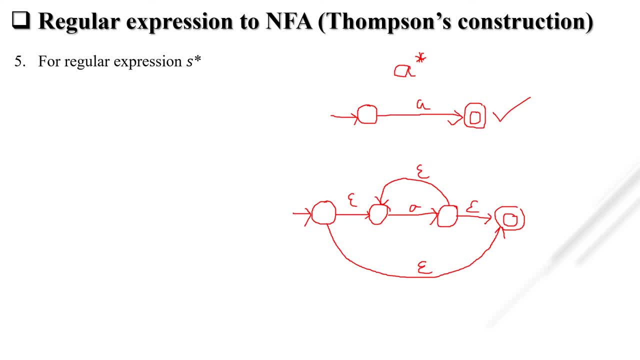 is a NFA for a star. it is very simple: what we were first to. we first draw the we were first to. we first draw the. we were first to. we first draw the NFA for a. then simply put one state at the NFA for a. then simply put one state at the. 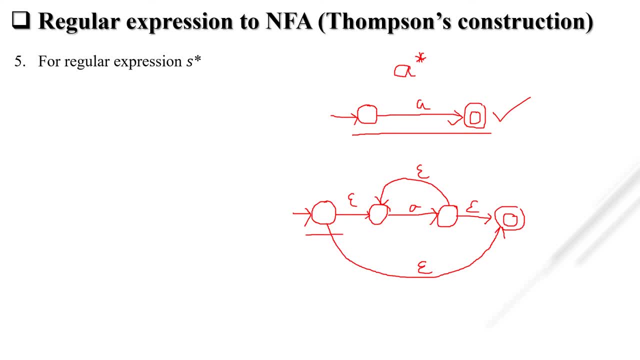 NFA for a. then simply put one state at the beginning of that NFA and the end of beginning of that NFA and the end of beginning of that NFA and the end of that NFA. okay, and there is a that NFA. okay, and there is a. 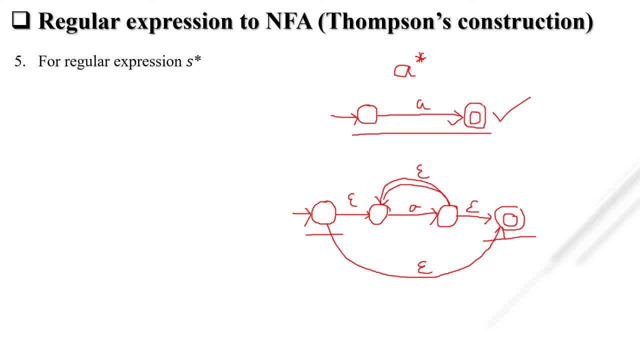 that NFA okay, and there is a transaction with null from ending state, transaction with null from ending state transaction with null, from ending state of a to the starting state of a, of a to the starting state of a, of a to the starting state of a to the starting state of a star, to ending state. 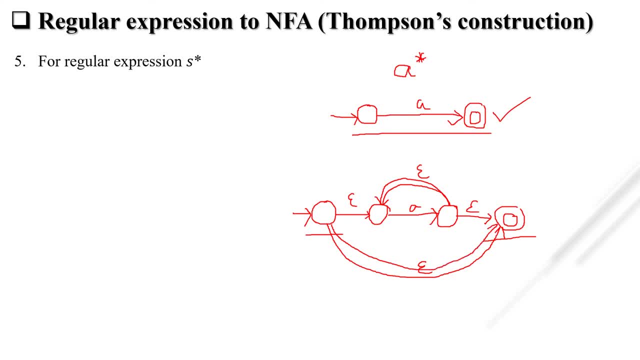 of a to the starting state of a star. to ending state of a. to the starting state of a star. to ending state of Easter. there is one of Easter. there is one of Easter. there is one directed arrow with with the symbol null. directed arrow with with the symbol null. 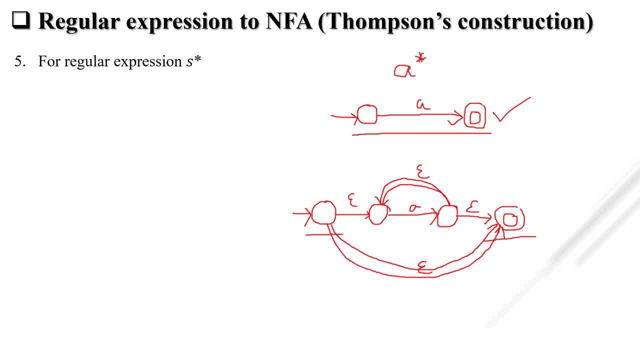 directed arrow with with the symbol null. okay, so let's see what is the NFA for a. okay, so let's see what is the NFA for a. okay, so let's see what is the NFA for a star. so, for example, there is a Easter. 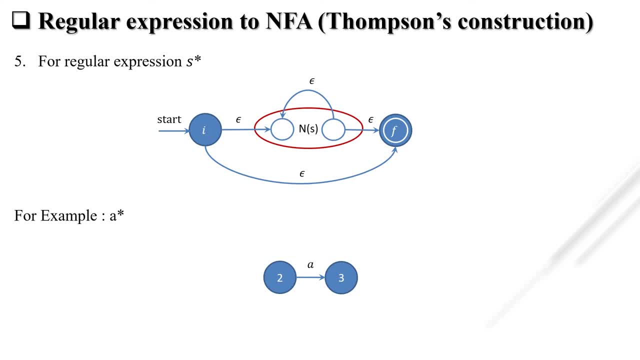 star. so, for example, there is a Easter star. so, for example, there is a Easter, then we have to drop first, and if a for, then we have to drop first, and if a for, then we have to drop first, and if a for, only a, then we have to. 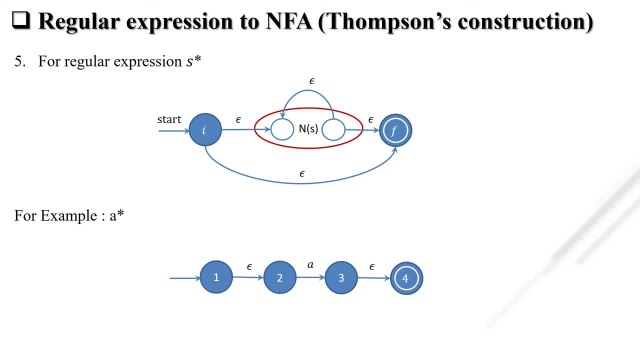 only a, then we have to drop first, and if a for only a, then we have to. then we have to drop first, and if a for only a, then we have to. then we have to drop first, and if a for only a, then we have to put one state at the beginning and one. 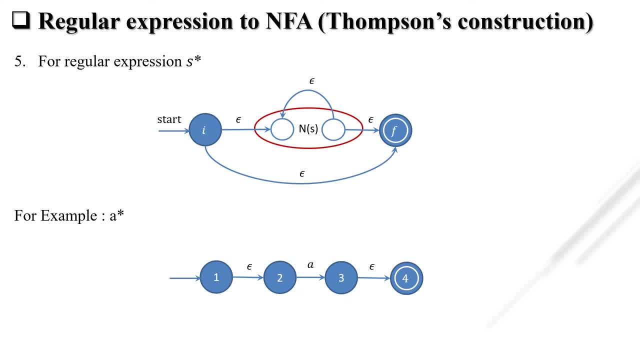 put one state at the beginning and one put one state at the beginning and one state at the end of the NFA. then we state at the end of the NFA, then we state at the end of the NFA, then we simply take the transaction from 3 to 2. 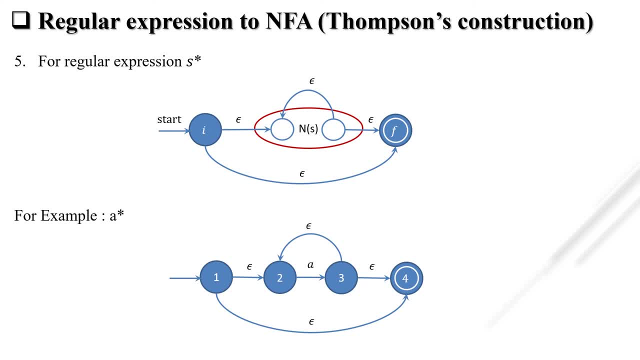 simply take the transaction from 3 to 2. simply take the transaction from 3 to 2 with the symbol null and the transaction with the symbol null and the transaction with the symbol null and the transaction from 1 to 4 with the time with the symbol. 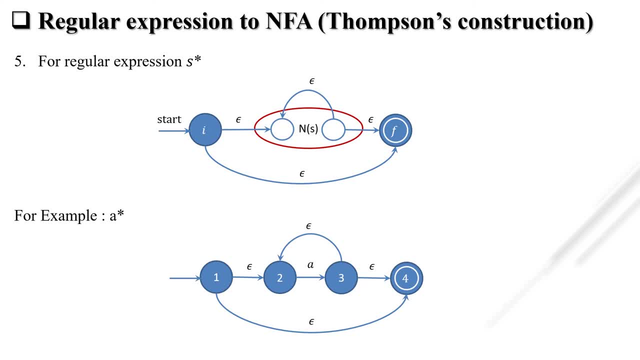 from 1 to 4 with the time with the symbol. from 1 to 4 with the time with the symbol. now, I hope you better understand so now. I hope you better understand so now. I hope you better understand. so, if there is a symbol, that a. 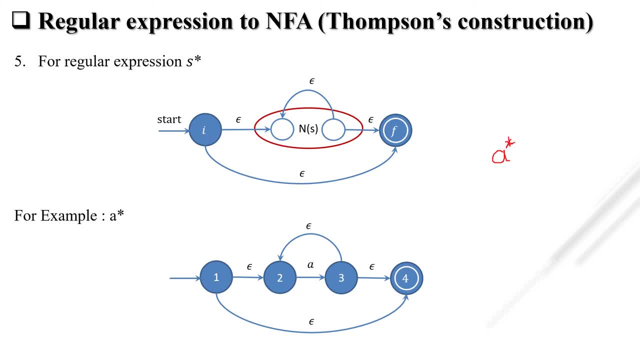 if there is a symbol that a, if there is a symbol that a star and B star, this is our, and you have star and B star, this is our, and you have star and B star, this is our, and you have to draw the NFA, then what you do, this is: 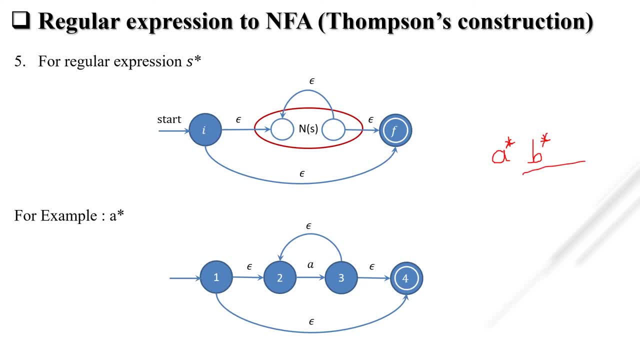 to draw the NFA, then what you do- this is to draw the NFA, then what you do, this is an initial state of whole B star. this is an initial state of whole B star. this is an initial state of whole B star. this is the initial state for whole B star. so we 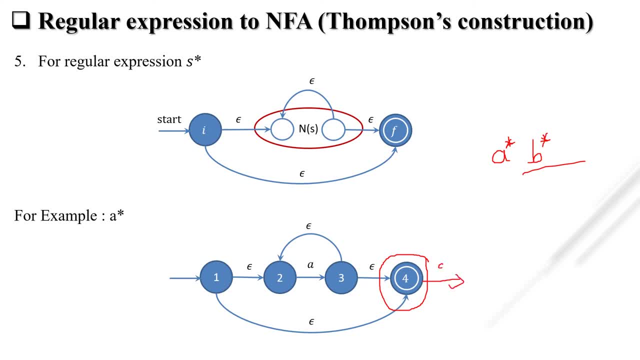 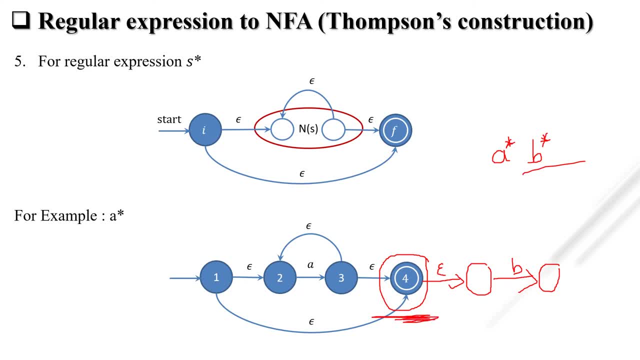 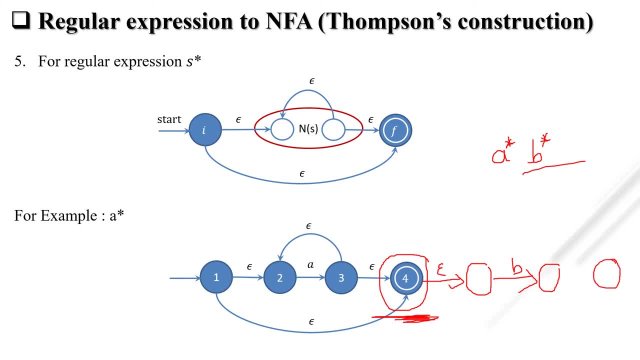 beginning of the NFA of B and at the end. beginning of the NFA of B and at the end of the NFA of B. okay with the symbol of the NFA of B, okay with the symbol of the NFA of B, okay with the symbol null, and we have to pass from the end. 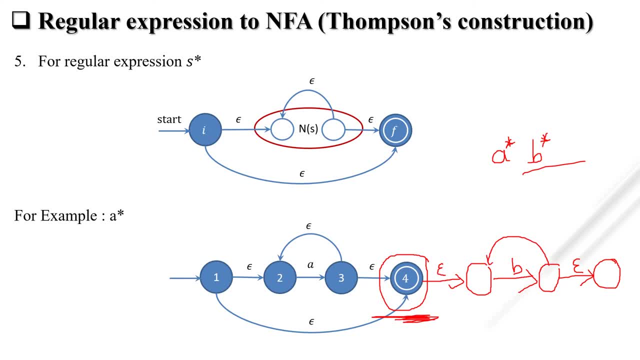 null and we have to pass from the end null and we have to pass from the end state to first initial state of B, with state to first initial state of B, with state to first initial state of B, with the symbol null and there is a: the symbol null and there is a. 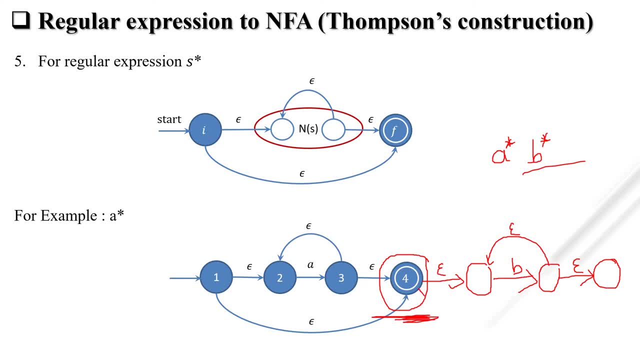 the symbol null and there is a transaction from initial state of B star. transaction from initial state of B star. transaction from initial state of B star to final state of V star. okay, so here as to final state of V star. okay, so here as to final state of V star. okay, so here, as we see in the regular expression, null. 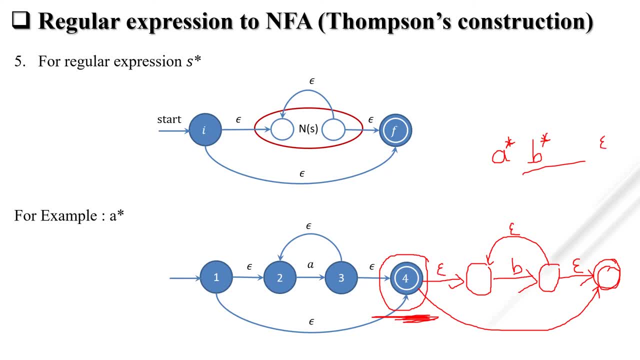 we see in the regular expression null. we see in the regular expression null string is also passed. okay, suppose I string is also passed. okay, suppose I string is also passed. okay, suppose I have a string null- nothing, then it is. have a string null- nothing, then it is. 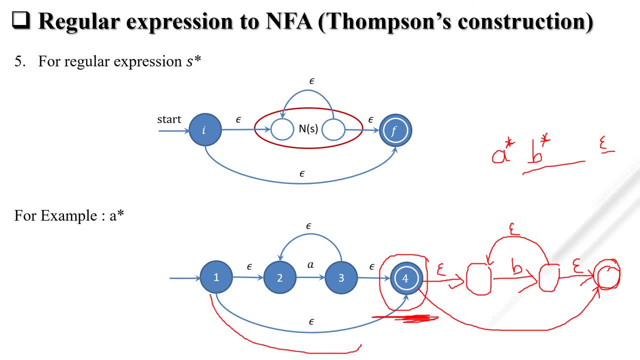 have a string- null, nothing- then it is also passed from null. we are to four, and also passed from null. we are to four, and also passed from null. we are to four. and then you have to this: it reaches to the. then you have to this: it reaches to the. 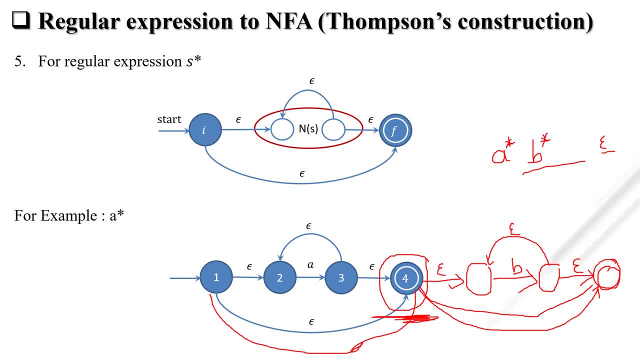 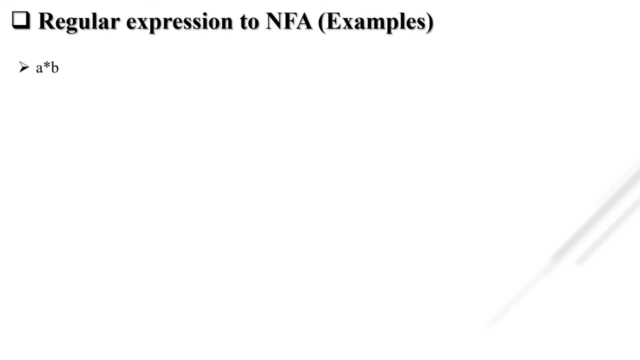 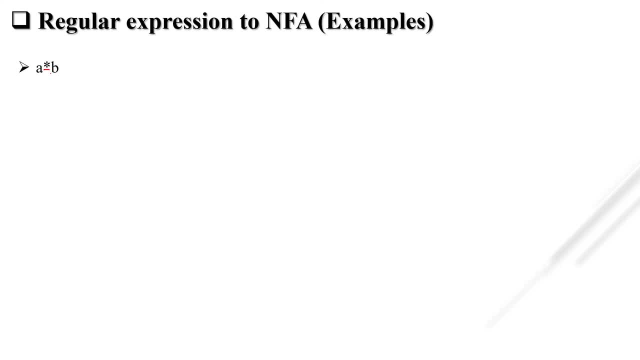 to star which is concatenate with B to star which is concatenate with B. okay, so, first what we do, we simply draw. okay, so, first what we do, we simply draw. okay, so, first what we do, we simply draw the NFA of a star that we already, the NFA of a star that we already. 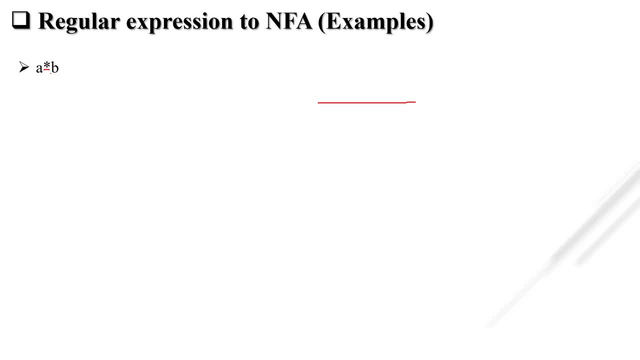 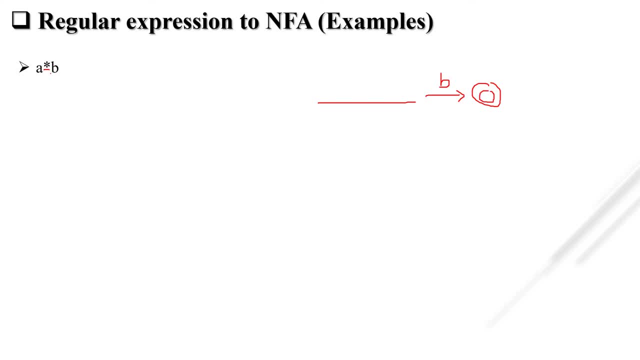 B. this is our final state. okay, so let's see the NFA. okay, so, let's see the NFA. okay, so let's see the NFA. first. we draw the NFA for only a star first. we draw the NFA for only a star first. we draw the NFA for only a star, then simply concatenate with B, which is: 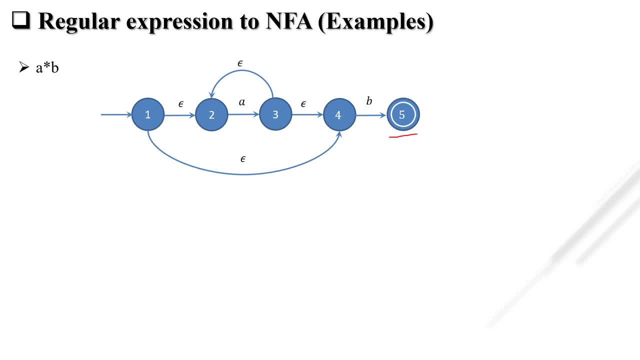 then simply concatenate with B, which is then simply concatenate with B, which is our final state. this phi is our final, our final state. this phi is our final, our final state, this phi is our final state. next b, star a, b, so first we. next b, star a, b, so first we. 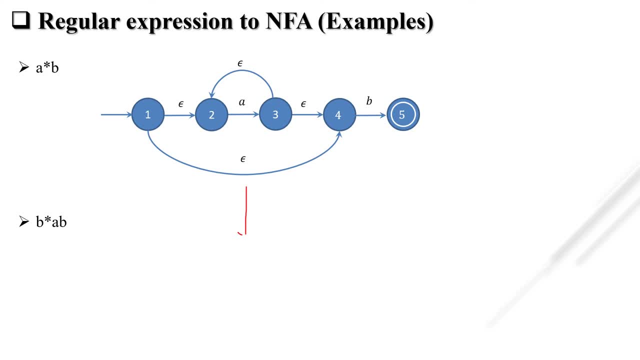 next b star, a, b. so first we similar to the, similar to the, similar to the. this a star. first we draw the NFA of B- this a star. first we draw the NFA of B- this a star. first we draw the NFA of B star and then concatenate with a, then B. 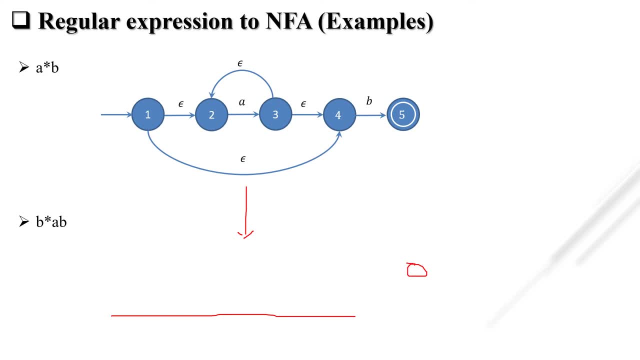 star, and then concatenate with a, then B star, and then concatenate with a, then B for a and B. what we do simply from first for a and B, what we do simply from first for a and B, what we do simply from first state, a from next state, this is and this. 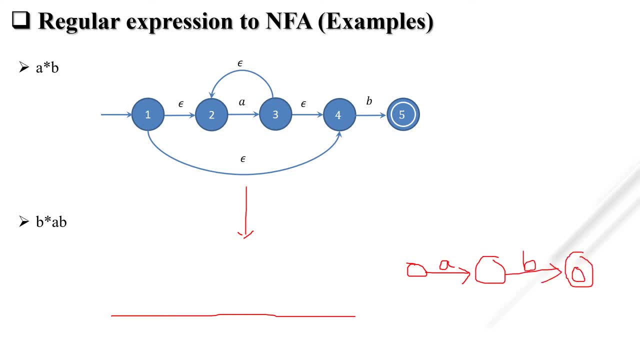 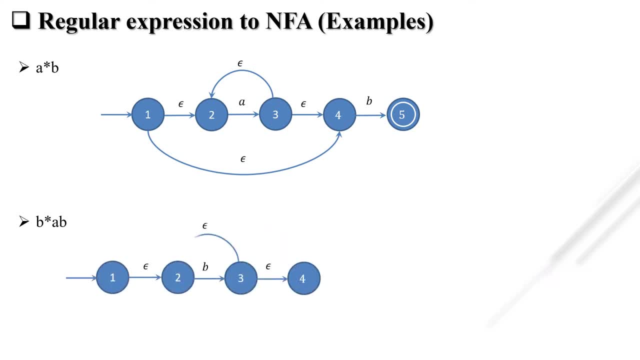 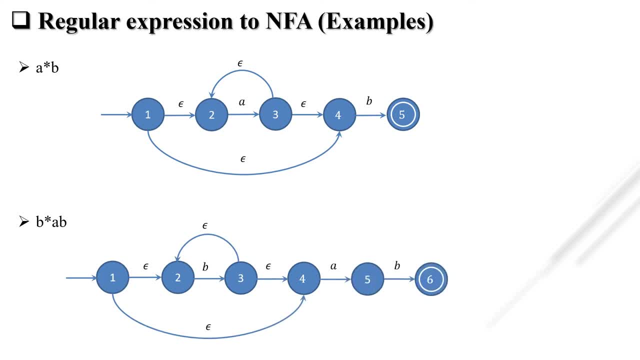 first we draw the NFA for B star, then concatenate with a, and then B and 6 is concatenate with a, and then B and 6 is concatenate with a, and then B and 6 is our final state. so the next and very our final state. so the next and very. 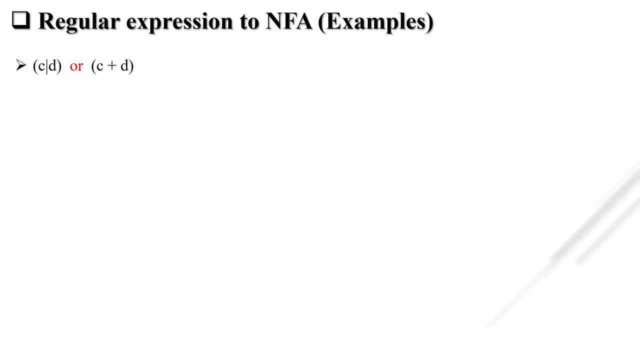 our final state. so the next, and very important, is C or D. it may be a or B, it important is C or D. it may be a or B. it important is C or D. it may be a or B, it may be 0 or 1. so for C or D, we already 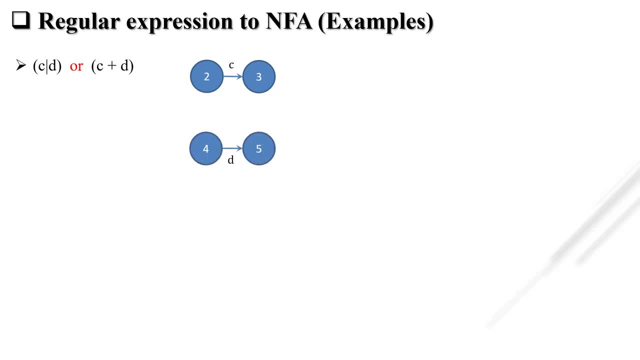 may be 0 or 1, so for C or D. we already may be 0 or 1, so for C or D. we already see in the previous slide that we we see in the previous slide that we we see in the previous slide that we we separate first C and D and then join with. 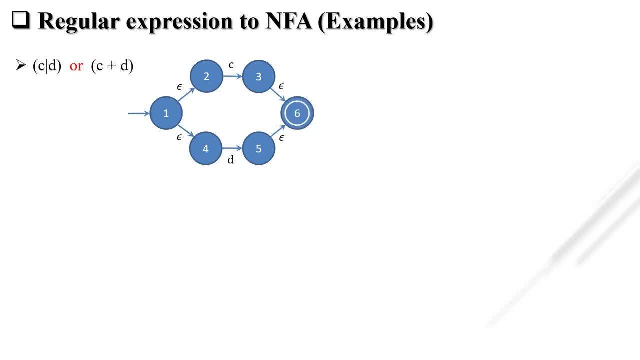 separate: first C and D and then join with separate: first C and D and then join with none. okay, the next one is C or D, the none. okay, the next one is C or D, the none. okay, the next one is C or D, the whole star now for a star. what we do, we? 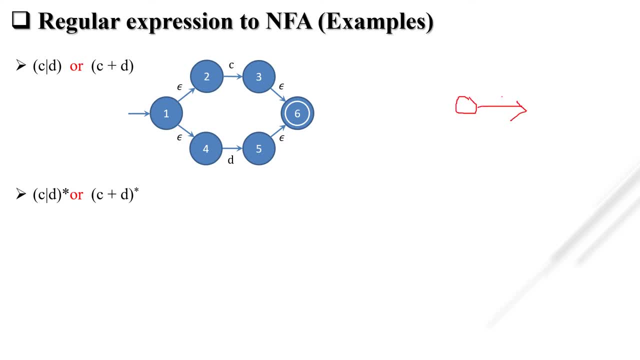 whole star now for a star. what we do we whole star now for a star. what we do? we simply have a transition of a from one, simply have a transition of a from one, simply have a transition of a from one state to another state. okay, then we add: 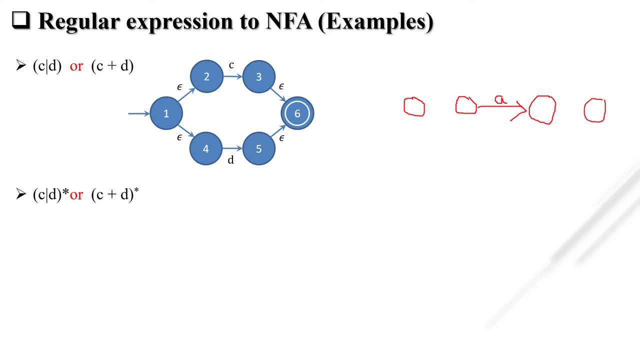 state to another state. okay, then we add state to another state. okay, then we add one state in the beginning and one state. one state in the beginning and one state. one state in the beginning and one state and the last, similarly for C or D, and the last, similarly for C or D. 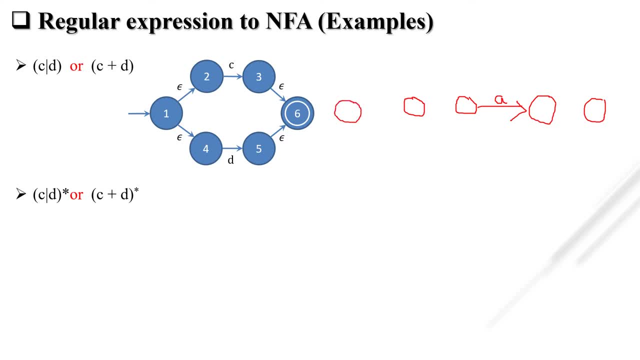 and the last. similarly for C or D. what we do, we would state at the last. and what we do, we would state at the last. and what we do, we would state at the last and at the beginning. okay in a what we at the beginning. okay in a what we. 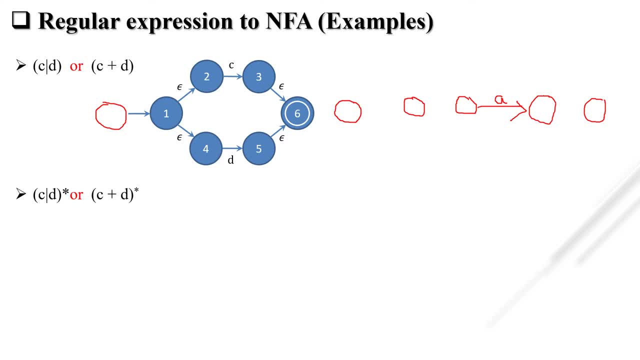 at the beginning. okay, in a, what we do from the final state of only a to the do, from the final state of only a to the do, from the final state of only a to the initial state of a. we have a directed initial state of a. we have a directed. 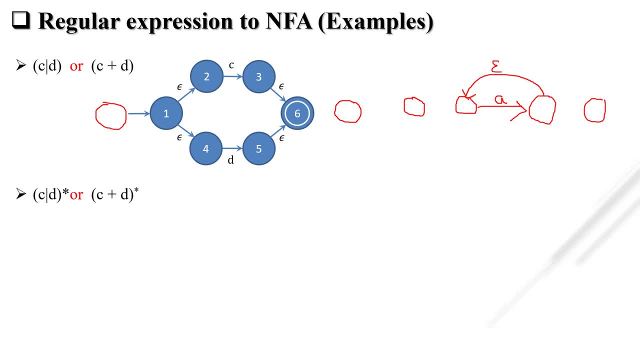 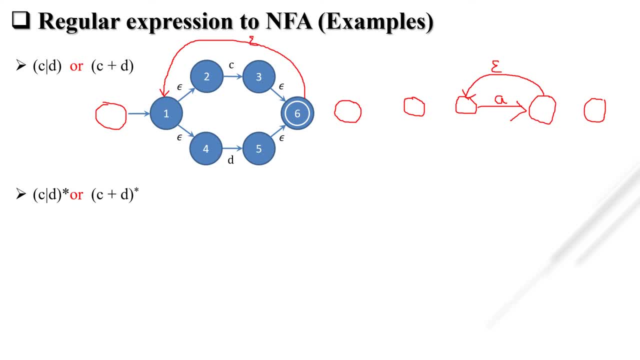 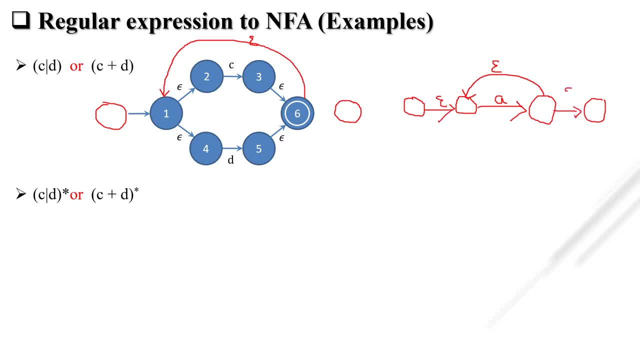 what we do, there is a null transaction. what we do, there is a null transaction. here, yeah, this is our final state. or here, yeah, this is our final state. or here, yeah, this is our final state. or initial state. from initial state to initial state, from initial state to. 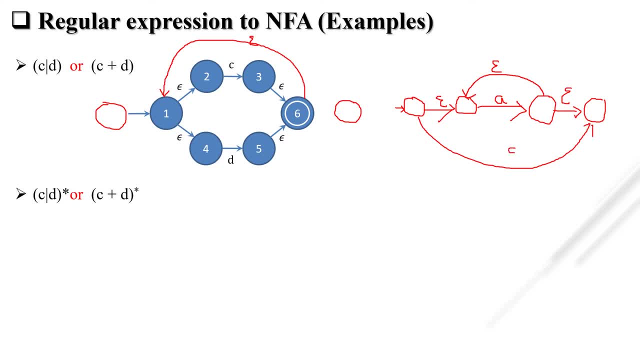 initial state, from initial state to final state. we have a transition of null final state. we have a transition of null final state. we have a transition of null. similarly in C or D, the whole star from. similarly, in C or D, the whole star from. similarly, in C or D, the whole star, from initial state to the final state. we. 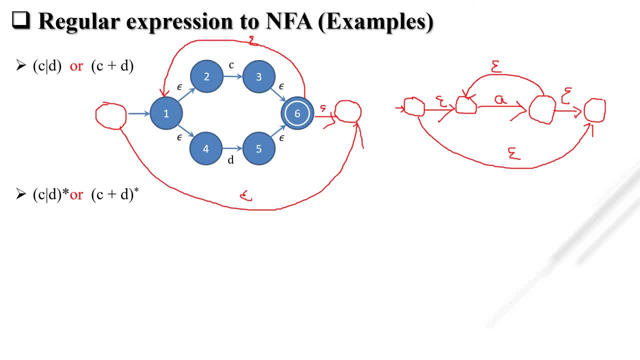 initial state to the final state. we initial state to the final state. we have a transition of, have a transition of, have a transition of is very simple. if you know the a star is very simple. if you know the a star is very simple. if you know the a star, then it is easy to draw the C or D, the 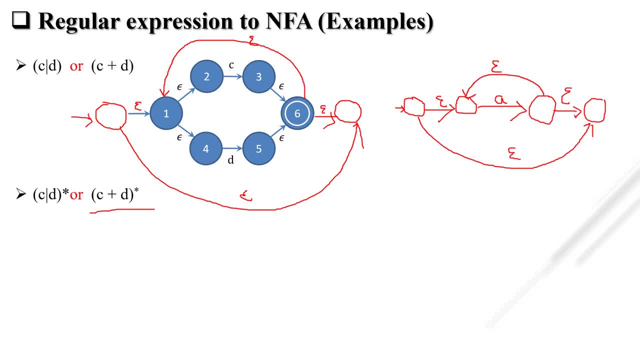 then it is easy to draw the C or D the. then it is easy to draw the C or D the whole star. this is our instance. okay, whole star, this is our instance. okay, whole star, this is our instance. okay, let's see the NFA first, we draw the. 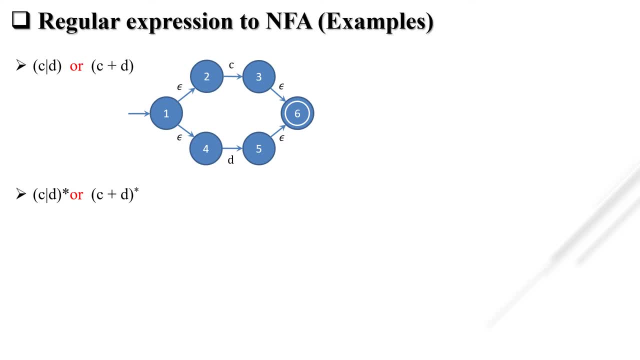 let's see the NFA. first we draw the. let's see the NFA. first we draw the NFA for only C or D, and then we add to NFA for only C or D, and then we add to NFA for only C or D, and then we add to state in the beginning and at the last. 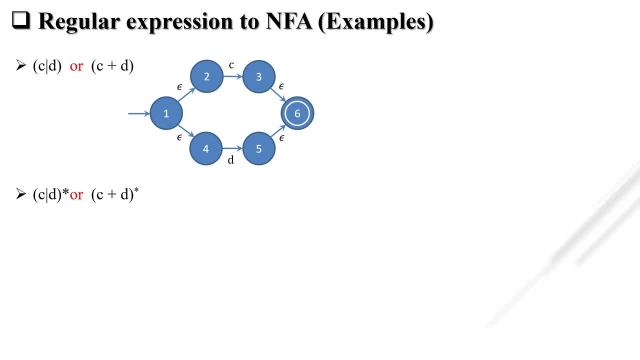 state in the beginning and at the last state in the beginning and at the last. okay. then there is a transition from. okay. then there is a transition from final state to the starting state of C or D, and then there is a transition of null from starting state to the final state of C or D. the whole star. okay, here null is also going to pass. how? 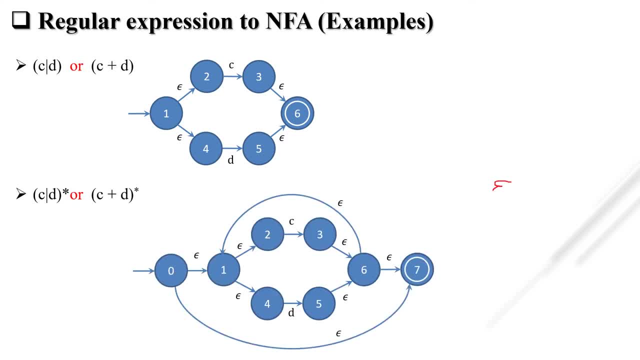 if you have a string null, then it will pass directly from initial state to final state. it is going to accept it. as we already see in the re, that null is also accepted in the cleans closure. so this exercise you have to do by your own if you have any query. 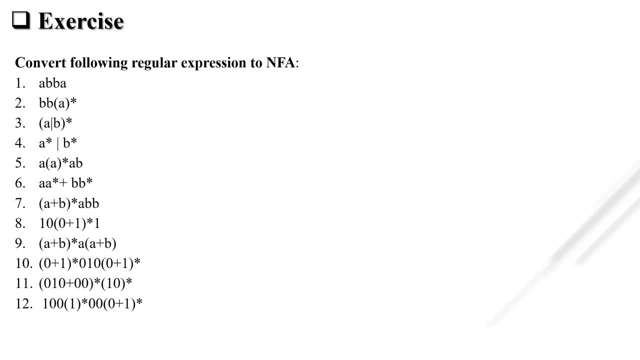 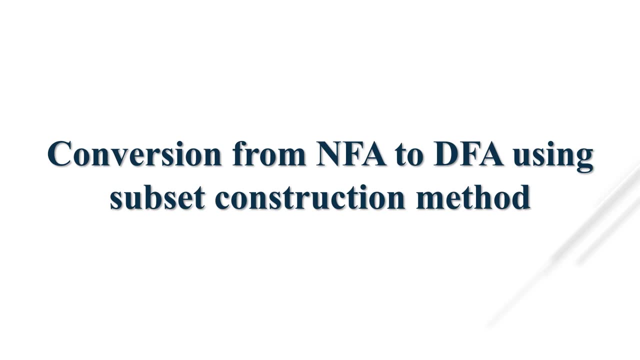 to constructing the NFA. please contact me, okay. so the next topic is conversion from NFA to DFA using subset construction method. in this you will see that the null is going to be accepted in the cleans closure. so this exercise you have to do by your own. if you have any query to constructing the NFA, please contact me okay. 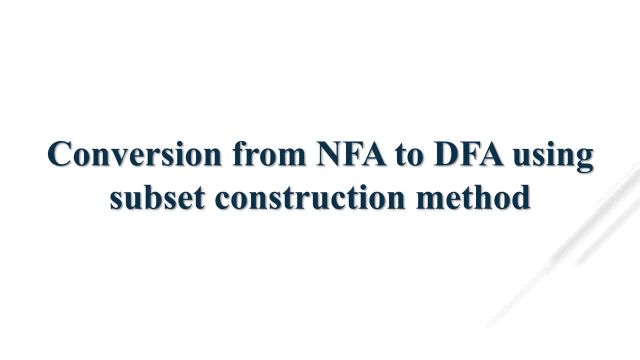 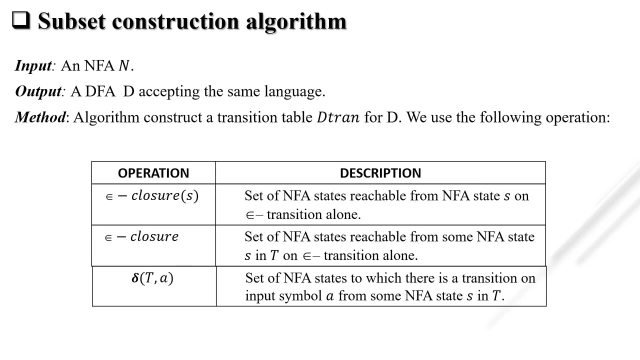 a topic re is already given. we have to form NFA using Thompson rule and then convert it into the DFA using subset construction method. so this is an algorithm for subset construction to perform a DFA from NFA. once we complete the example, then read this algorithm step by step. you will clearly understand. 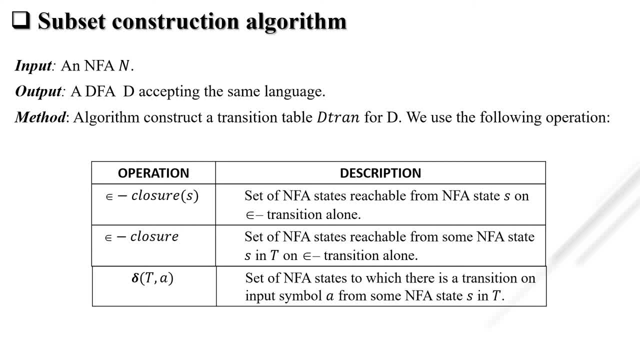 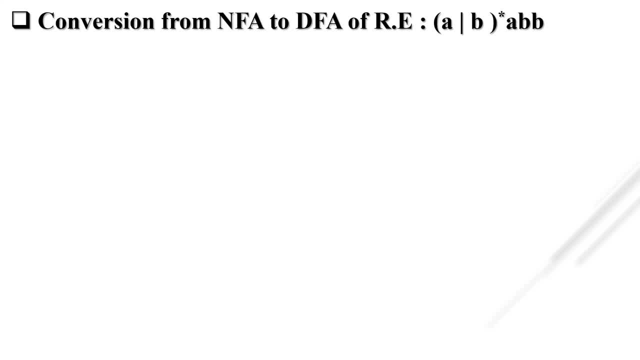 the algorithm. let's begin with the example first. so here we convert NFA to DFA using subset construction method for the re a or be the whole star a BB. so what is our first step? construct NFA for the re a or be the whole star a BB using Thompson rule, as we already know how to draw a. 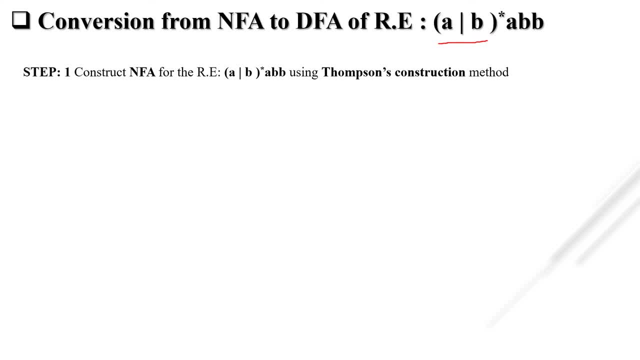 the NFA for a or B. so first we draw NFA for a or B and then for cleans closure. what we do we simply put one state at the beginning of the a or B and one state at the end of the a or B, okay, and then we concatenate this: a, then B and B. 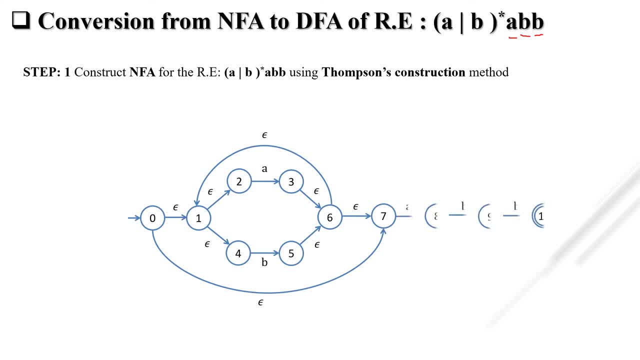 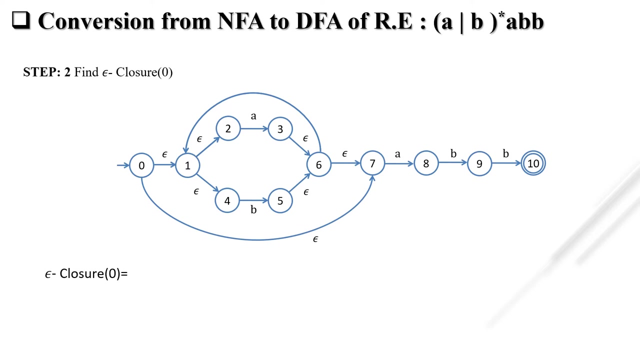 directly without including null. okay, and then we concatenate this a, then B and B directly without including null, and this is our final standard is 10 and 0 is our initial state. now let's see how subset construction method works to construct DFA. so the first step is to 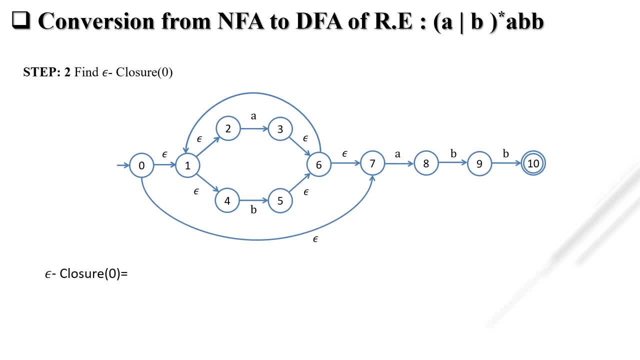 draw NFA and the second step is to find null closure of 0. if our initial state stated as 1, then we have to find null closure of 1. suppose you are giving the number from 1, then 2, then 3 and 4, so you have to find first null closure of. 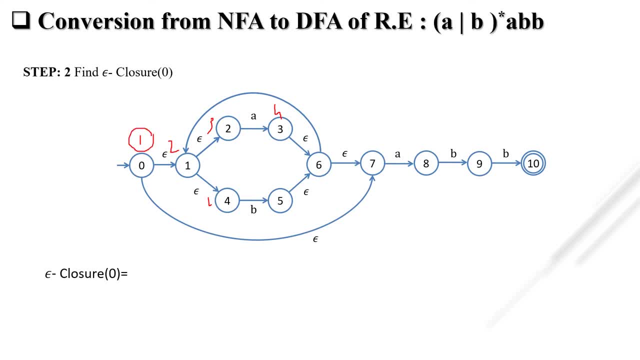 initial state, that is 1. here our initial state is stated as 0. that's why we are finding null closure of 0. so in subset construction method first we have to find null closure of initial state. here our initial state is 0, so we find: 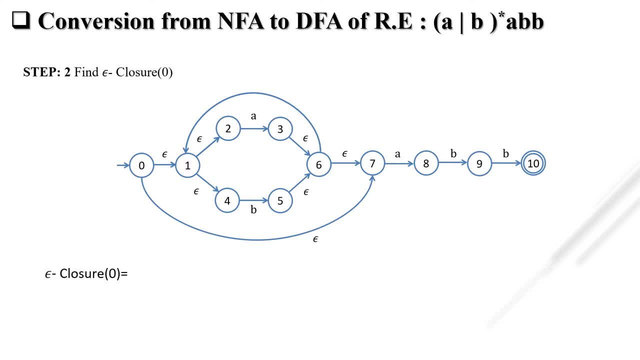 null closure of 0 first. so whenever we find null closure of any state, that state itself is a part of null closure. suppose, if I find null closure of the 1 and 2, so 1 and 2 is a part of the null closer and then the remaining one. okay, 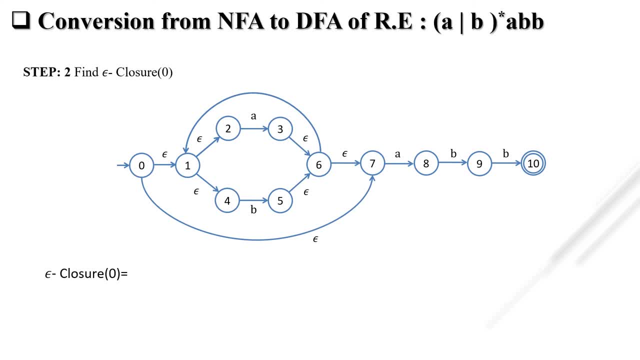 so let's see how to find the null closer of 0. so the null closer of 0 is 0 itself first, then from 0, the edges with the symbol null directly or indirectly stated, to next state. then it is a part of our null closer of 0. for example, from 0 to 1, there is a 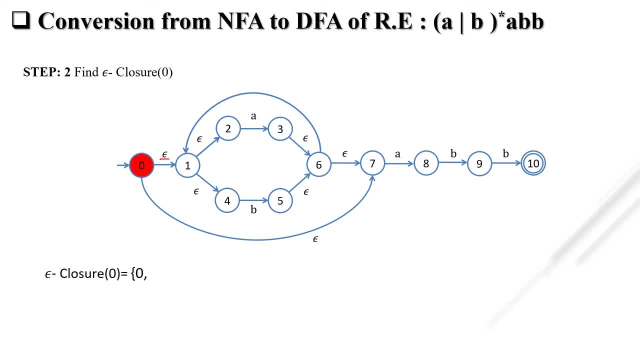 edge with null. so 1 is a part of null closer of 0. also from 0 to 7. it is a. it is a. there is a transition of null directly from 0 to 7. it may be indirectly or directly, okay, so 1 and 7 will be there. so from 0 to 1 and 1 to 2 and 4. 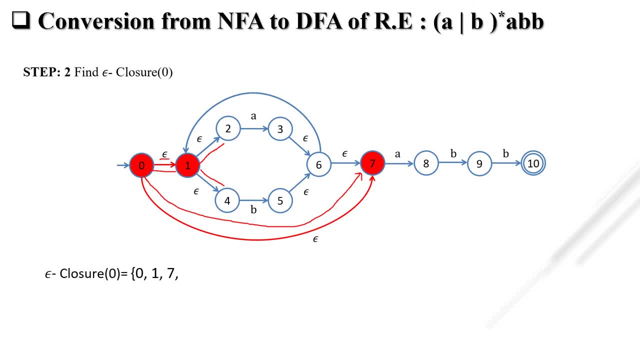 there is a transition from 0 to 2 by null. okay, we can consider null null as a single null. so 2 and 4 is also a null closure of 0. okay, from 7, there is no null leaving out to any state. from 2, also, no null is leaving out. 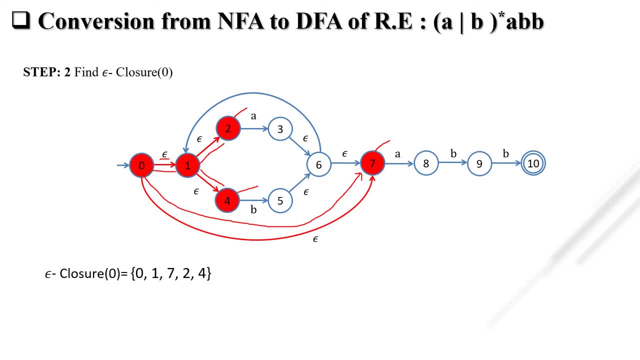 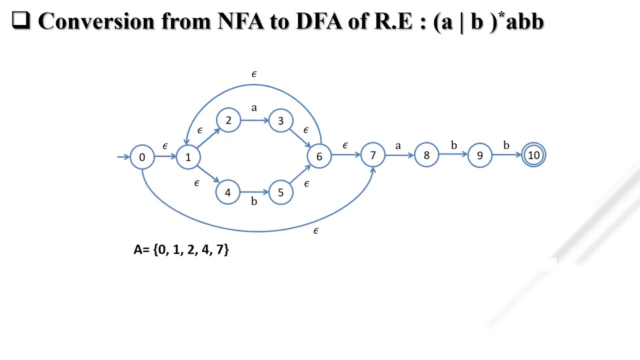 to any state from 4 also. so this is our null closure of 0. let us give the name is 0, 1, 7, 2 and 4 to a. okay, okay. so the next step is to find the transition of capital A of the input. 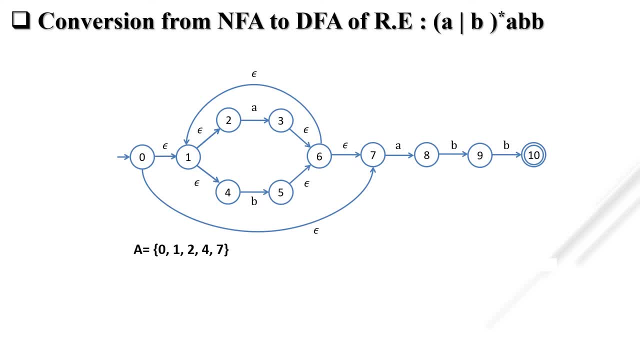 symbol that is small a and small b. so if there is a another symbol, that is C, then we have to find transition of a of a, a of B and a of C. but in re we have only two symbols, a and B. so we are only, we are going to find only the transition. 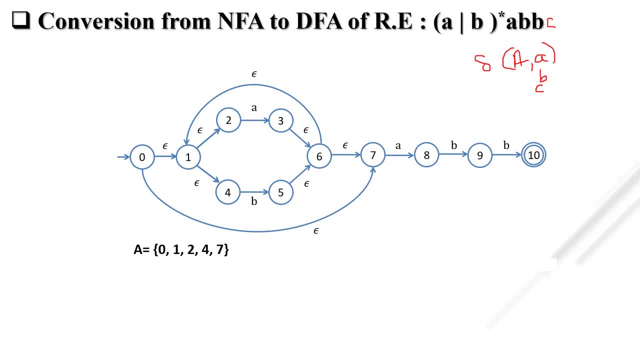 function of a of a and a of B. okay, so first we find the transition of capital, a of small a. what is our a? it is 0, 1, 2, 4 and 7. now we check this symbol that is small. a is living out. 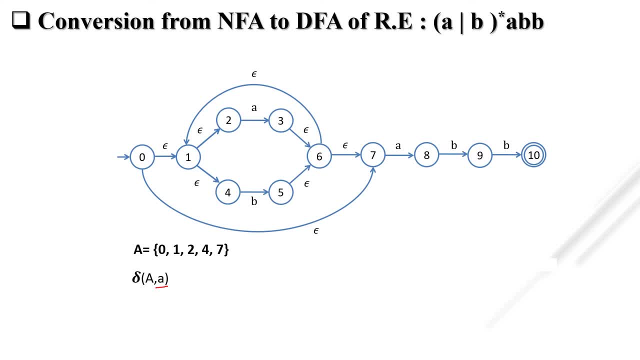 from any of these state. yes, from 2 it is directly reached to 3- okay. and also from 7 it is directly reached to 3- okay. and also from 7 it is directly reached to 3. it is directly reached to A. So here we are not going to check that A is directly or indirectly. 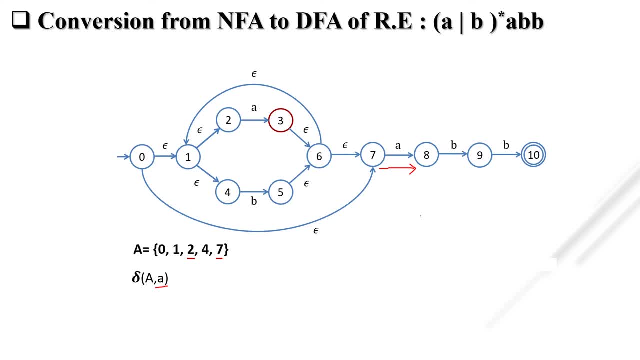 reaches to another state or not, In null what we do? We also considered the indirectly state also. For example, if I find the null closure of 0 and if this transition is null and this transition is also null, So what is the null closure of 0? 0,, 1 and 2.. 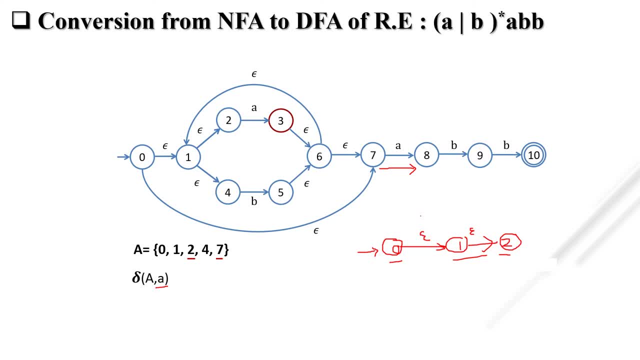 Okay. but when we find the transition of any state, then we check that this A is leaving out from any of this state. A is leaving out from 2 to 3 directly. So what is our answer? First, 3. Okay, then from 7 to 8, it is directly reaches. from 7, it is directly reaches to 8.. That's why I write. 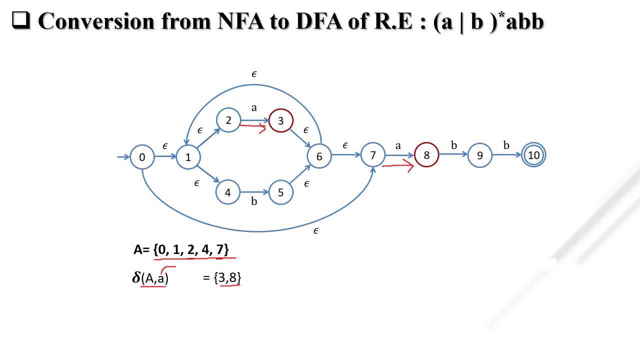 8 here. Okay, so don't consider this. from 0 also, it is reached to 3.. Okay, So the next step is to find the null closure of this 3 and 8.. So 3 and 8 is a part of this null closure, as we discussed earlier. 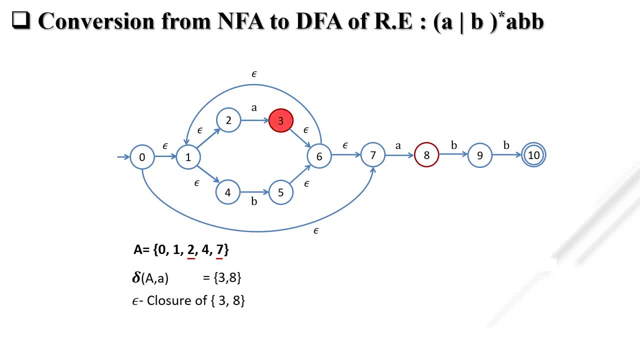 So what is the null closure of 3 and 8?? First 3 will be there. Then, by taking the null transaction, it reaches to 6.. Then it reaches to 1.. It reaches to 2 and 4.. It also reaches to 7.. What is the null closure of 8 itself? Why? Because from 8 there is no edges. 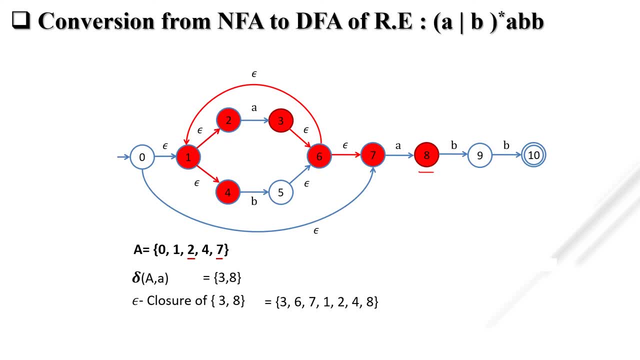 with symbol null reaches to any other state. Okay, so we label this as a- B. Why? Because A and B is not similar. If A and B is- both answer is similar- then we simply label this state as A, As it is not. 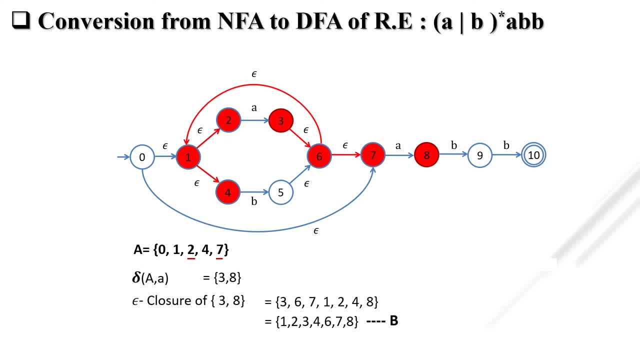 similar. we are labeled as a state b, so this is a transition table from a to a. what is our answer? b. what i write? simply b. so what is our next step? to find the transition function of a of b? what, um, whichever is the answer we simply put here: if there is a, c, if there is a or b, okay, 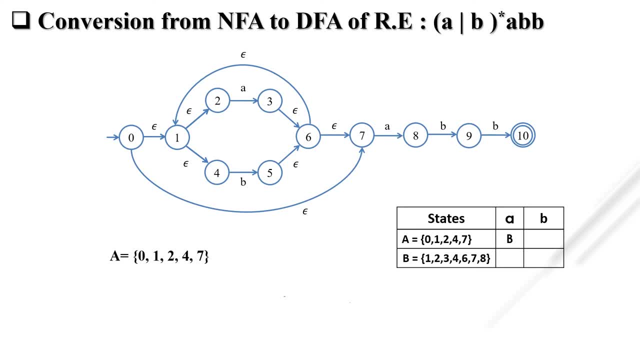 okay, now we find the transition function of a of b. so what is our? a? zero, one, two, three, and the answer is c. zero, one, two, three, and the answer is c: zero, one, two, three, and the answer is c to 4 and 7. now we check from 0. there is a directly transaction of b. is there no from 1? no from 2, no. 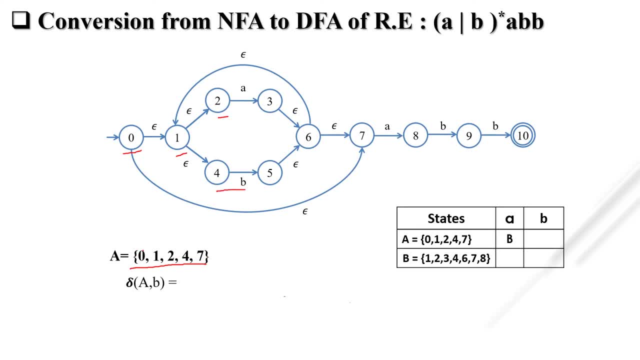 from 4, there is a directly transition to state 5. so what is our answer? 5. then from 7, is there is any transition of the symbol b? no, so what is our answer? only this: 5. now, the next step is to find null closure of 5. i is already there. from 5, there is a null transition. 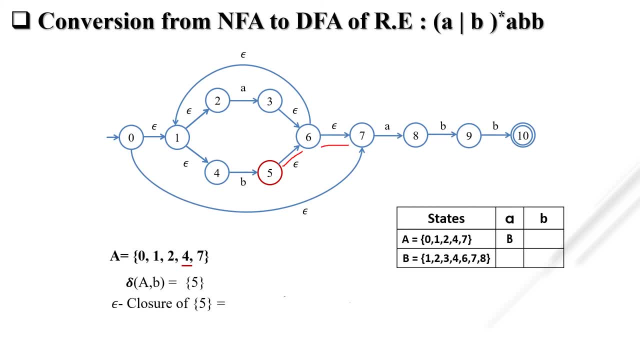 to 6 and 7, then from 6 to 1 and from 1 to 2 and 4. so what is the answer? 5, 6, 7 and 1, 2 and 4. okay, so is it similar to a or b? no, this is completely new state. 1, 2, 4, 5, 6, 7. here: 0, 1, 2, 4, 7. 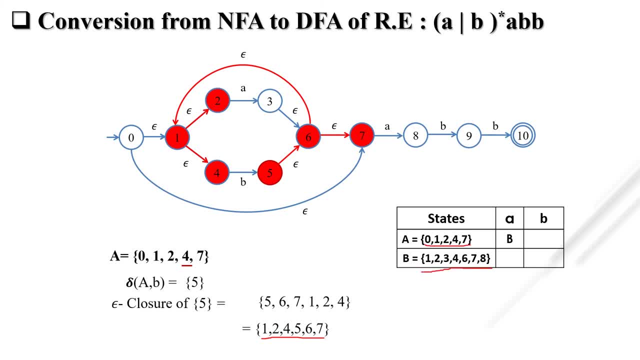 here: 1, 2, 3, 4, 6, 7. so we are going to label this as a state c. so what is transition of capital? a of b, that is c. so what is our answer? c. now we have one another state that is c. now we have to find b as we complete. 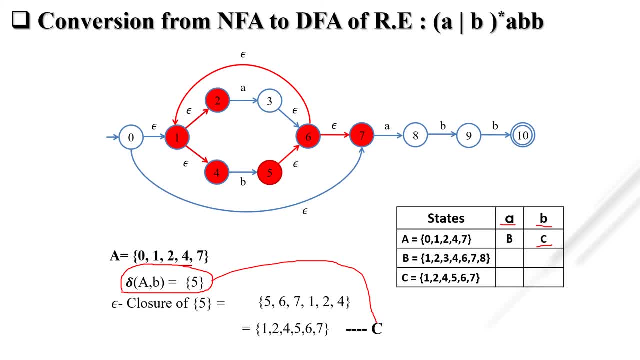 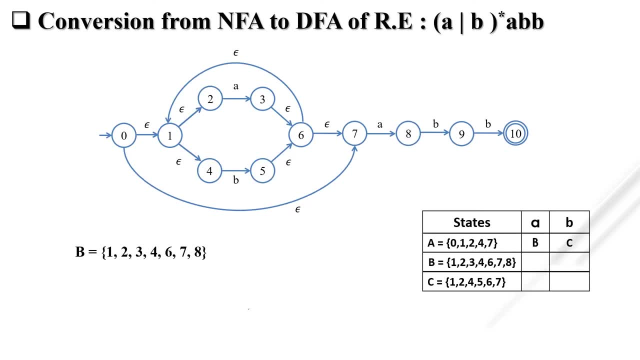 a of a and a of b. now we have to find b of a and b of b, okay. so here we are going to find b of a and b of b. so here we are going to find b of a and b of b, to find transition of b of a and b of b. so first we find b of a. what is our b? 1, 2, 3, 4, 6, 7 and 8. 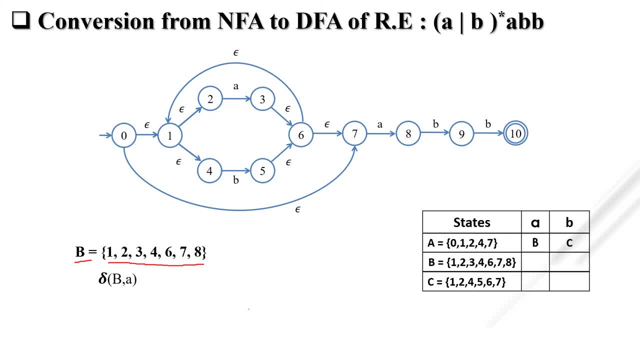 now we check: is there any transaction directly reaches to any state with the symbol a from 1? there is no directly. it is with a. is reached to any other state from 2? yes, it reaches to 3, 3. so what is our answer? first 2, sorry, 3. next, from 3: is there any transaction with the symbol a? no, 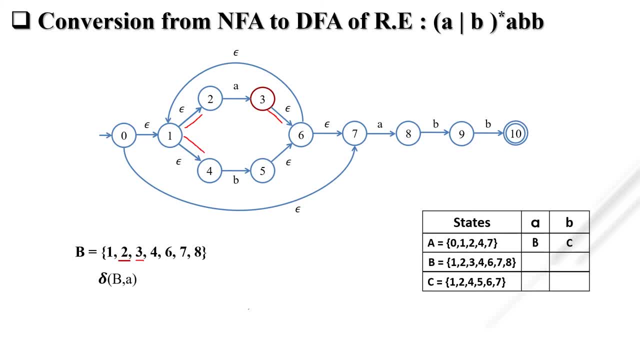 then 4: no, and from 7: yes, there is a directly transition of a to the state 8. so what is our answer? next, 8 from 8: no, there is no transition of a to any other other state. so what is the answer? 3 and 8. so what is our next step? we have to find null. closure of 3. 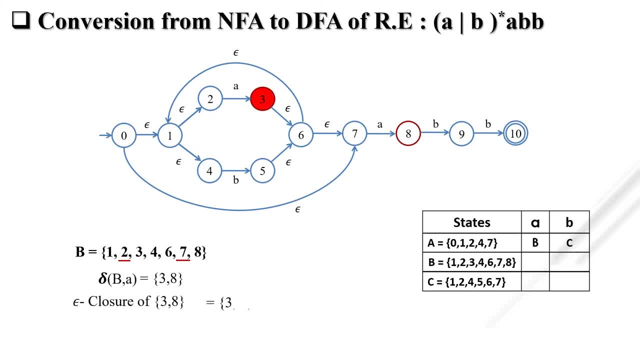 and 8. what is the null closer of 3 and 8? first 3, then it reaches to 6, then it reaches to 7, 1, 2 and 4 and it will be the part of this null closure. so, as you see, one, two, three, four, six, seven and eight it. 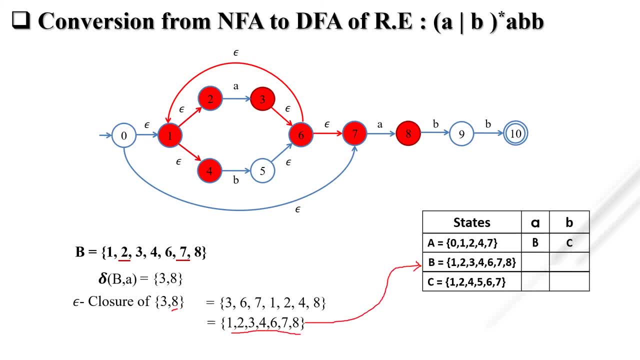 is already already there, okay. so we are not going to label this state as a, as a D, we have to label this state as a, B. so what is the transition of B of a? what is our answer? B. so what? we are right, B, okay. so next we are going to find transition. 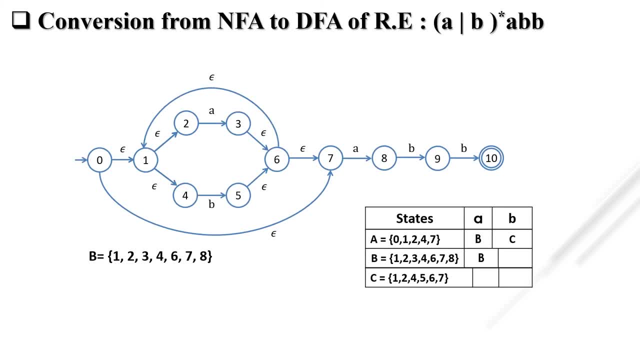 of B of B, so from four, Disney, it is directly transition of B to five. so by I raised our answer. from six there is no transition of B. from seven there is no transition of me. from eight there is a directly transitional B to the state nine. so nine is our. 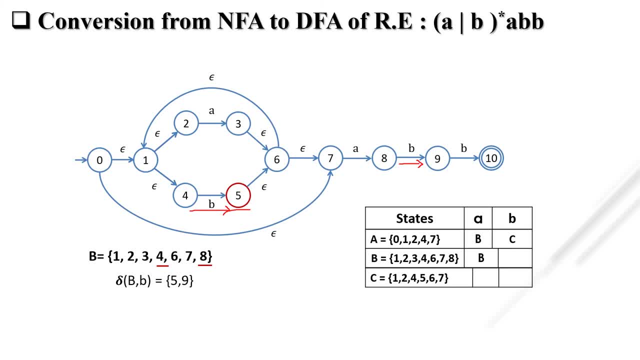 answer: 5 and 9. so what is our next step? we have to find null closure of 5 and 9. 5 and 9 is the part of this null closure, so 5 is already there. from 5 there is 6, then 7, 1, 2 and 4. 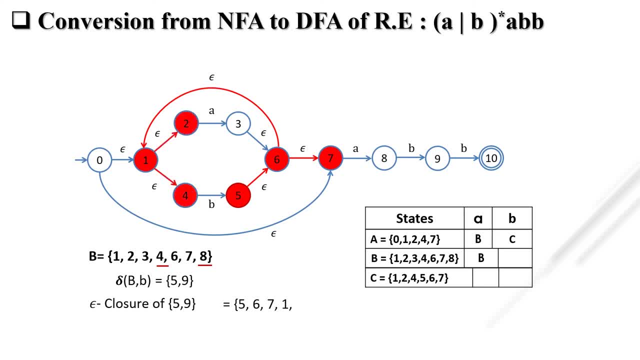 okay then what is the null closure of 9 9 itself? there is no edges with the symbol. null is reaches to other state. okay, so this is a new state. so we have to label this state as a d and also insert in the transition table. okay. 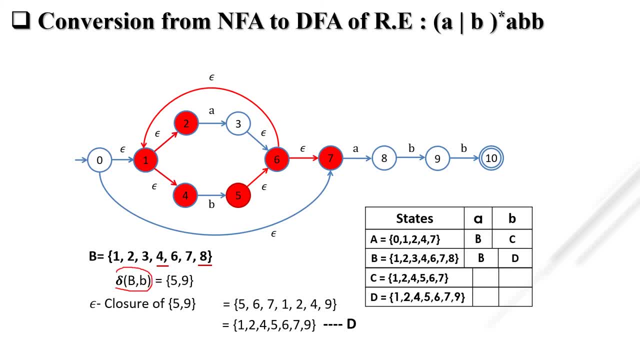 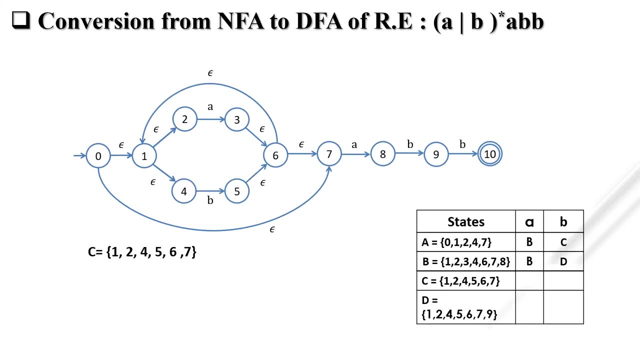 okay, okay, okay, okay, okay. so transition of capital B of B. what is the answer? small, sorry: capital D, so we write here D. so here we already complete the state A and B by finding transition of A of A, A of B and B, of A and B of B. now next one is C, so we have to find transition function of C of A and C of B. 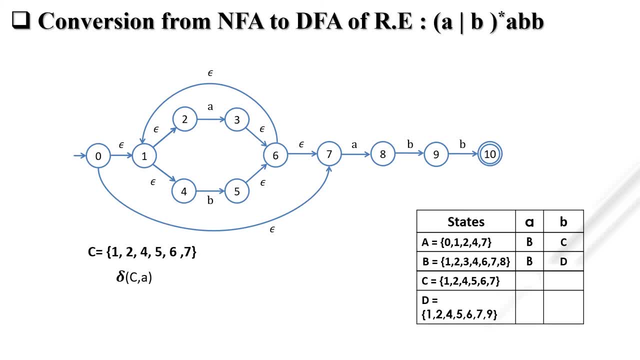 now next one is C, so we have to find transition function of C of A and C of B. now next one is C, so we have to find transition function of C of A and C of B. so what is the transition of C of A from the state to the edges, leaving to the state 3 with the symbol a. so 3 is the answer. 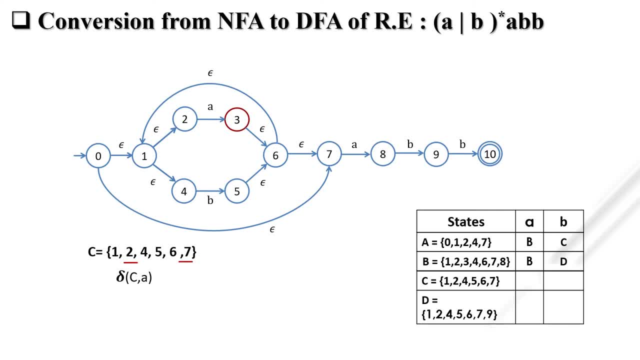 next from 7, there is a directly edges with the symbol a, which is reaches to the state 8. next, from 7, there is a directly edges with the symbol a, which is reaches to the state 8. next, from 7, there is a directly edges with the symbol a, which is reaches to the state 8. so what is our answer? 3 and 8 from 1, 4, 5 and 6. 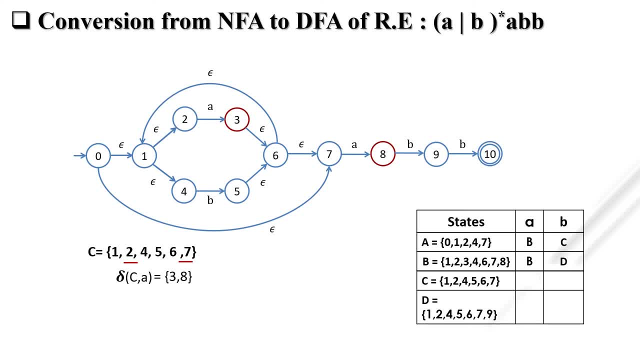 so what is our answer? 3 and 8 from 1, 4, 5 and 6. so what is our answer? 3 and 8 from 1, 4, 5 and 6? there is no edges living out with the symbol a. there is no edges living out with the symbol a. 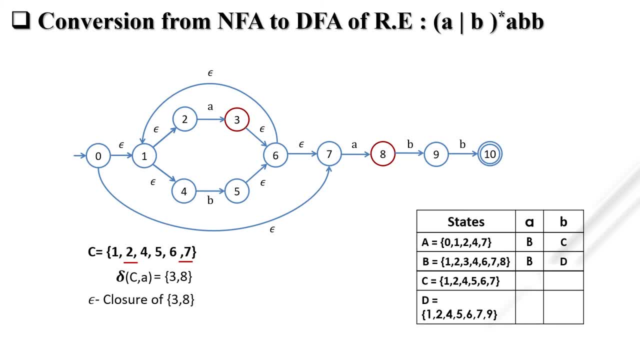 there is no edges living out with the symbol a. okay, so next step is to find null closure of. okay, so next step is to find null closure of. okay, so next step is to find null closure of 3 and 8. what is null closure of 3 and 8? 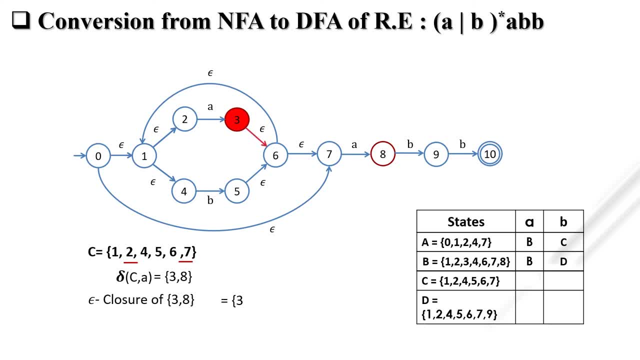 3 and 8. what is null closure of 3 and 8? 3 and 8, 3 itself, 3 itself, 3 itself, then from 3 to 6, then from 3 to 6, then from 3 to 6, then 1, 7. 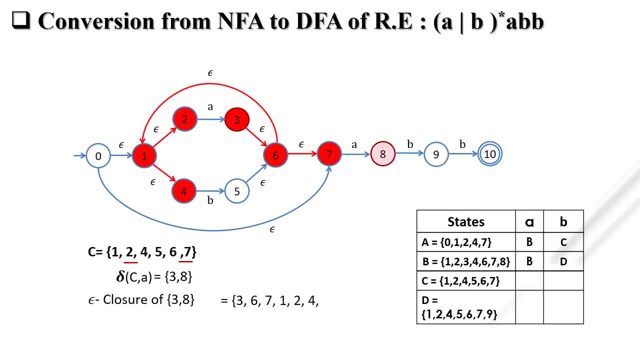 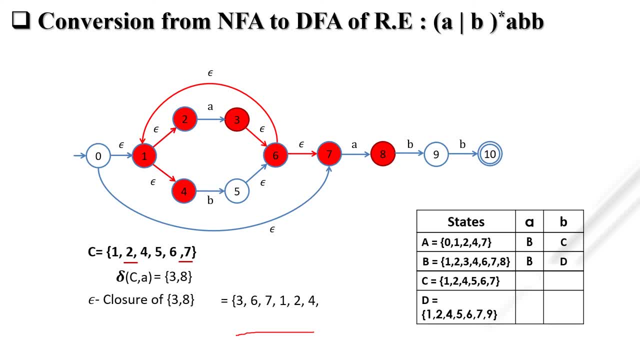 this state is already there. it is 1, 2, 3, 4, 6, 7. it is 1, 2, 3, 4, 6, 7 it, so we are not 4, 6, 7. it is 1, 2, 3, 4, 6, 7 it, so we are not. 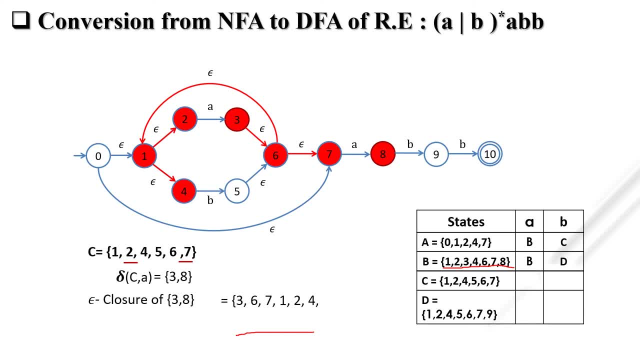 4, 6, 7. it is 1, 2, 3, 4, 6, 7 it. so we are not going to label with the new state. we going to label with the new state. we going to label with the new state. we simply put the state B, okay, so the 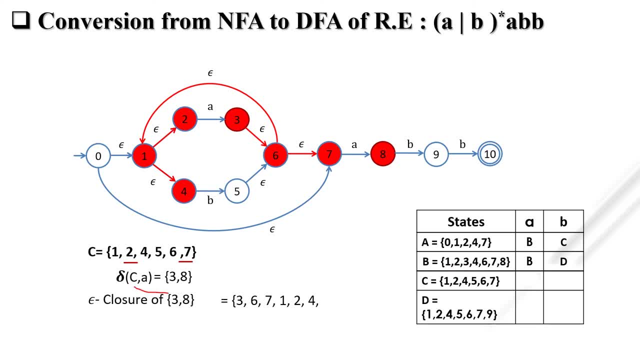 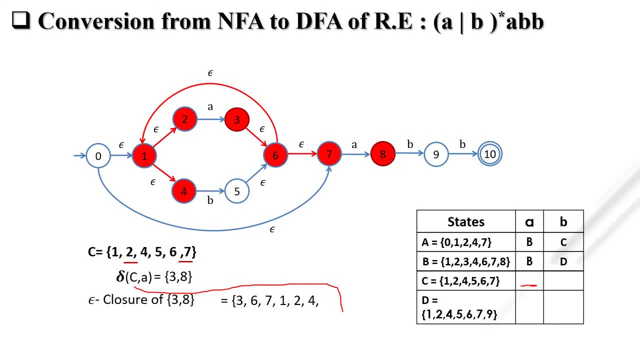 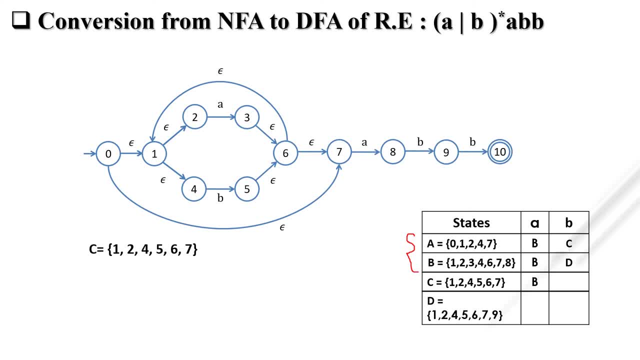 function of C of. we already find a of a function of C of. we already find a of a, a of B and B of a, B of B, and also we a of B and B of a, B of B, and also we a of B and B of B, and also we find C of a. now we have to find transition. 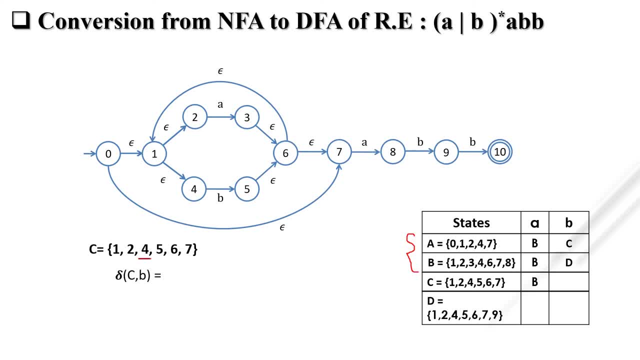 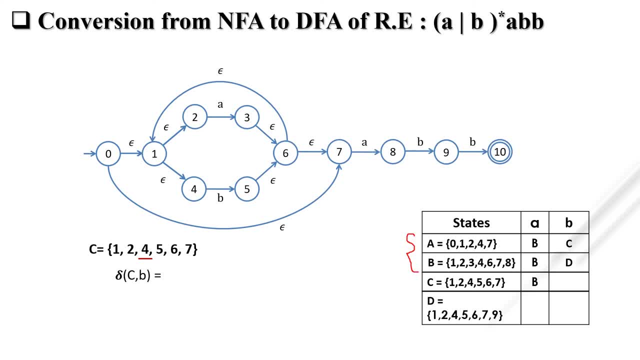 there is no, there is no. it is living out with the symbol B from. it is living out with the symbol B from. it is living out with the symbol B from: 2 also from 4. there is a age living out. 2 also from 4. there is a age living out. 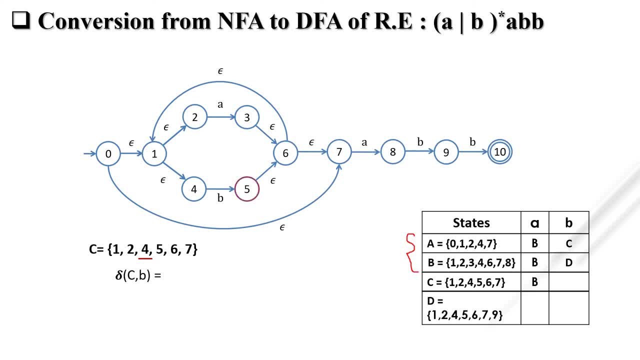 2, also from 4. there is a age living out. with B to 5. what is our answer? first one with B to 5. what is our answer first one with B to 5. what is our answer? first one is 5 from 5. there is no edges living out. 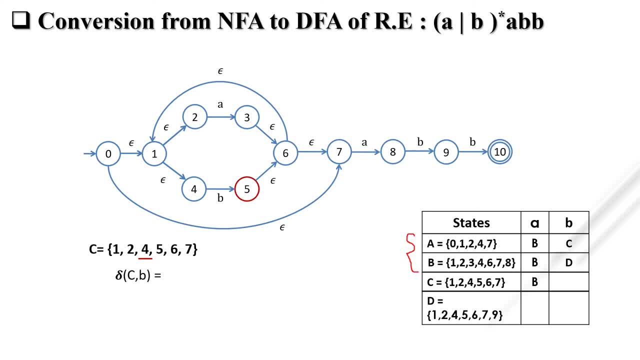 is 5 from 5. there is no edges. living out is 5 from 5. there is no edges. living out with the symbol B from 6, also from 7, also, with the symbol B from 6, also from 7, also, with the symbol B from 6, also from 7 also. so only 5 is our answer. what is the? 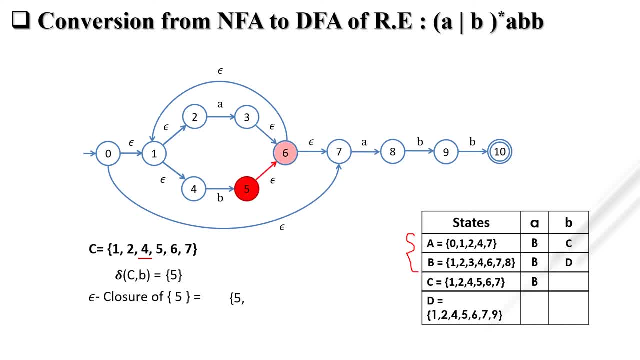 so only 5 is our answer. what is the? so only 5 is our answer. what is the closer of 5? 5 itself in 6, 1 and 7, 2 and 4? closer of 5: 5 itself in 6, 1 and 7, 2 and 4? 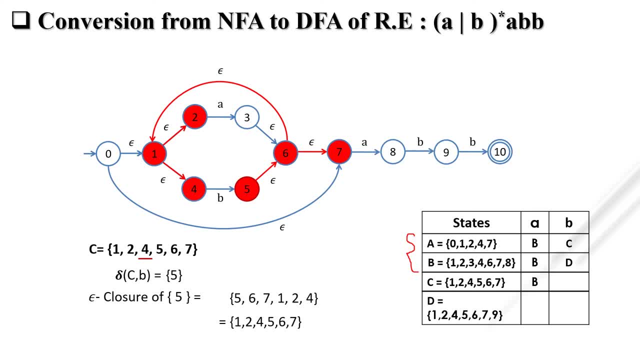 closer of 5, 5 itself, in 6, 1 and 7, 2 and 4. so this state is already. we find it is 1, so this state is already. we find it is 1, so this state is already. we find it is 1, 2, 4, 5, 6 & 7: 1, 2, 4, 5, 6 & 7. so what we? 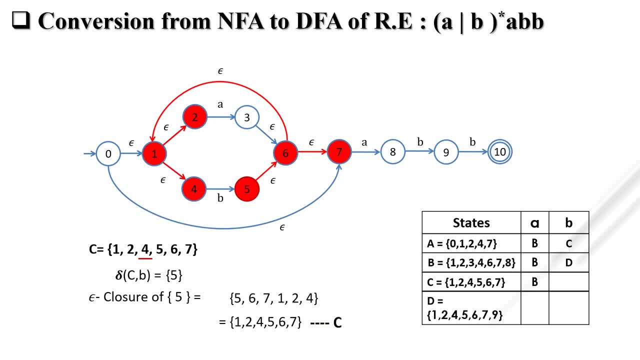 2, 4, 5, 6 & 7. 1, 2, 4, 5, 6 & 7. so what we? 2, 4, 5, 6 & 7. 1, 2, 4, 5, 6 & 7. so what we level this? we label this state as a C. 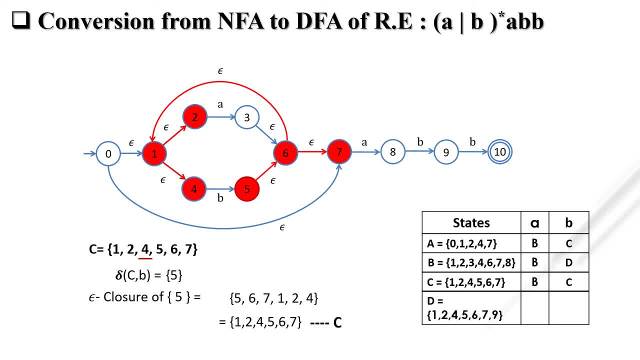 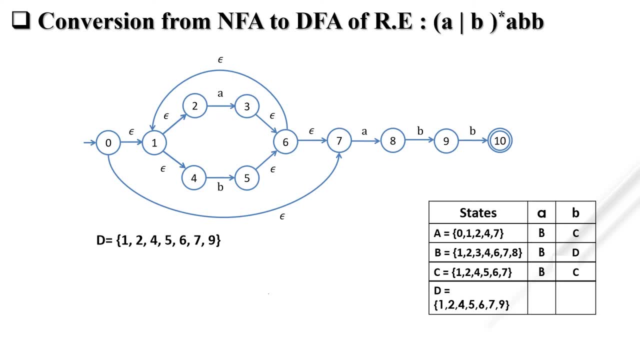 level, this state as a C level, this state as a C, and also insert C of B as a C- now we have- and also insert C of B as a C- now we have- and also insert C of B as a C- now we have to find, to find. 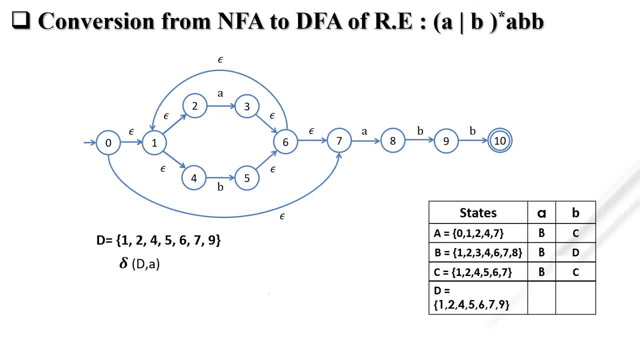 to find transition of D of a. what is d? 1, 2, 4, 5, 6, 7? transition of D of a. what is d? 1, 2, 4, 5, 6, 7? transition of D of a. what is d? 1, 2, 4, 5, 6, 7 & 9? from 1? there is no transition of a. 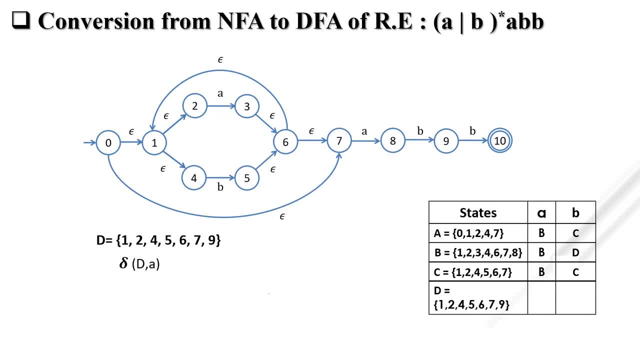 & 9 from 1. there is no transition of a & 9 from 1. there is no transition of a from 2. there is a transition of a to the from 2. there is a transition of a to the from 2. there is a transition of a to the state. 3 from 4. there is no transition of. 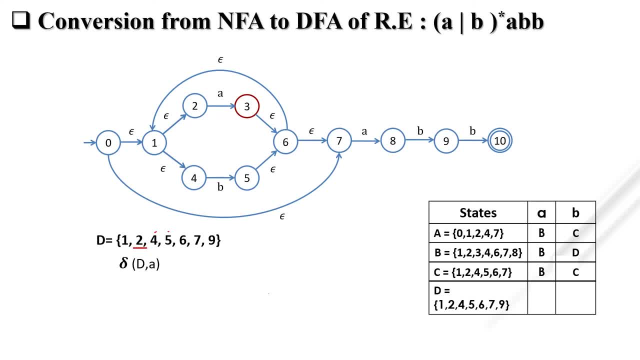 state 3 from 4. there is no transition of state 3 from 4. there is no transition of a from 5. there is no transition of a from a from 5. there is no transition of a from a from 5. there is no transition of a from 6. there is no directly transition of a. 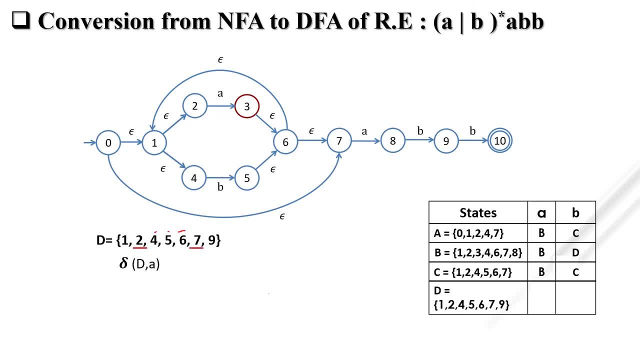 6. there is no directly transition of a from 6. there is no directly transition of a from 7. there is a transition of a to the from 7. there is a transition of a to the from 7. there is a transition of a to the from 9. there is no transition of the. 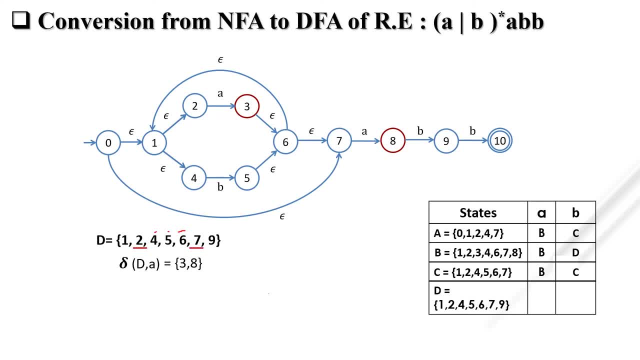 from 9, there is no transition of the. from 9, there is no transition of the symbol a. so what is our answer? 3 & 8, symbol a. so what is our answer? 3 & 8, symbol a. so what is our answer? 3 & 8. next, we have to find null closure of 3. 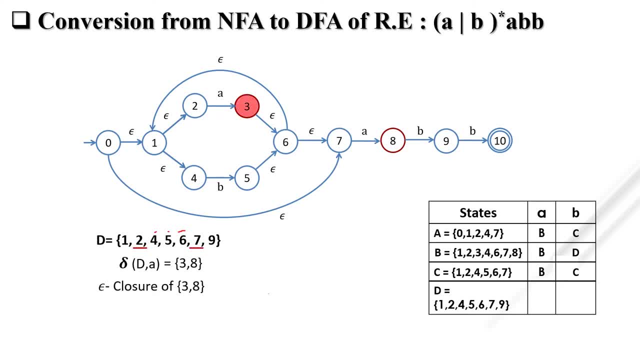 next we have to find null closure of 3. next, we have to find null closure of 3 & 8- 3. null closure of 3 is 3 itself, then & 8- 3. null closure of 3 is 3 itself, then & 8- 3. null closure of 3 is 3 itself, then 6, then 7 & 1 & 2 & 4. what is the null? 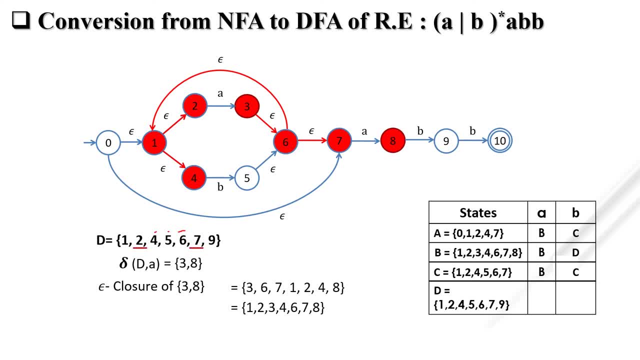 6, then 7 & 1 & 2 & 4. what is the null? 6 then 7 & 1 & 2 & 4. what is the null? closure of 8, 8 itself. so 1, 2, 3, 4, 6, 7, 8. 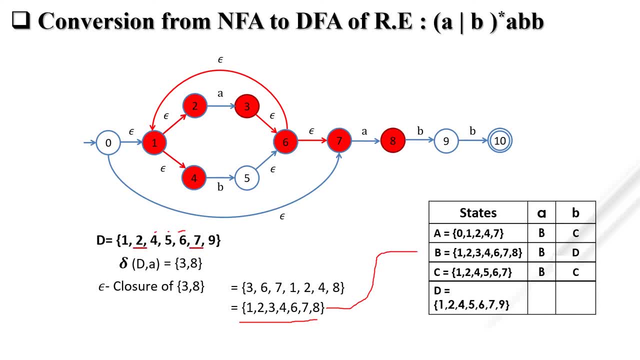 closure of 8- 8 itself. so 1, 2, 3, 4, 6, 7, 8. closure of 8- 8 itself. so 1, 2, 3, 4, 6, 7, 8. it is already there, so we are not going. 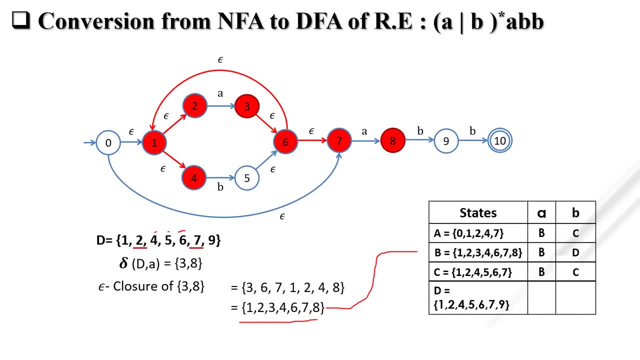 it is already there, so we are not going. it is already there, so we are not going to label this as a new state. simply put to label this as a new state. simply put to label this as a new state. simply put capital B. okay, so del of transition. 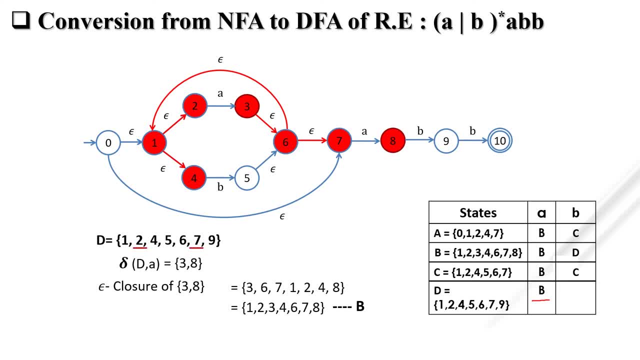 capital B. okay, so del of transition capital B. okay, so del of transition function of D of a is B. next now we function of D of a is B. next now we function of D of a is B. next now we have to find transition function of D. 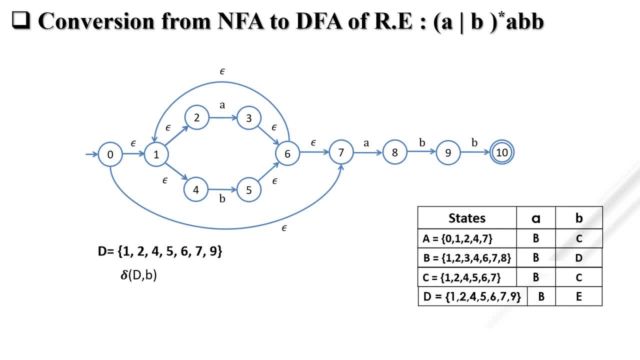 have to find transition function of D, have to find transition function of D of B. so from 1 there is of B, so from 1 there is of B. so from 1 there is no transition of B from 2, also from 4. no transition of B from 2, also from 4. 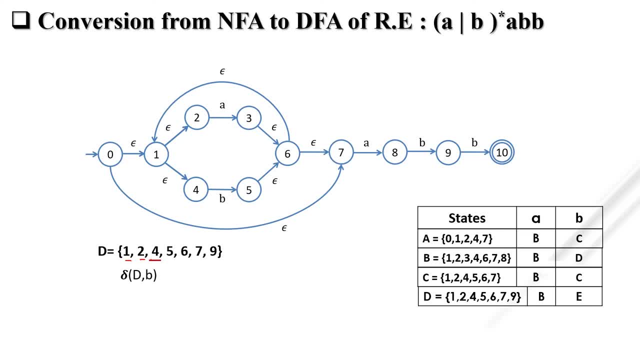 no transition of B from 2, also from 4. there is a transition of B which reaches. there is a transition of B which reaches. there is a transition of B which reaches to the state 5. over is our a, 5 is our. to the state 5. over is our a, 5 is our. 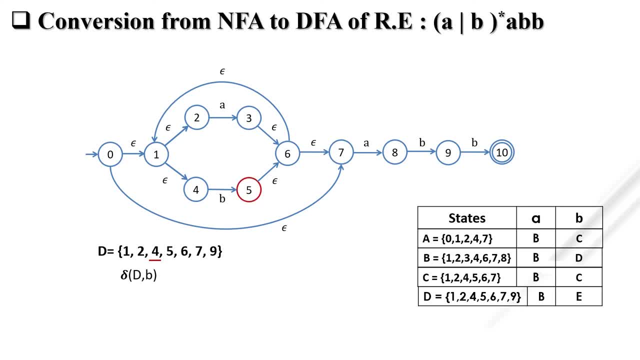 to the state: 5 over is our a, 5 is our answer. then from 5, there is no answer. then from 5: there is no answer. then from 5: there is no transition. of B. from 6: there is no transition of B from 6: there is no. 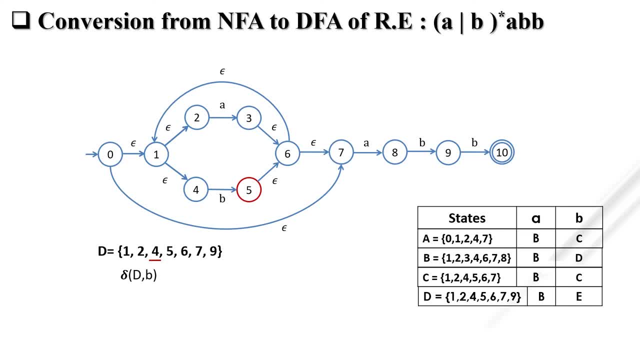 transition of B from 6. there is no transition of me from 7. there is no transition of me from 7. there is no transition of me from 7. there is no transition of you from 8. there is a transition of you from 8. there is a. 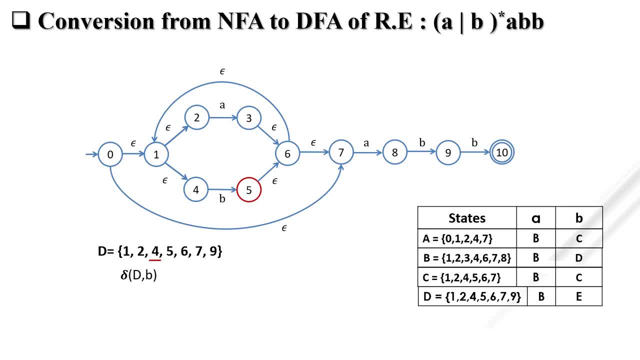 transition of you. from 8 there is a transition of you, but 8 is not in our transition of you. but 8 is not in our transition of you, but 8 is not in our state D. so from 9 there is a transition state D. so from 9 there is a transition. 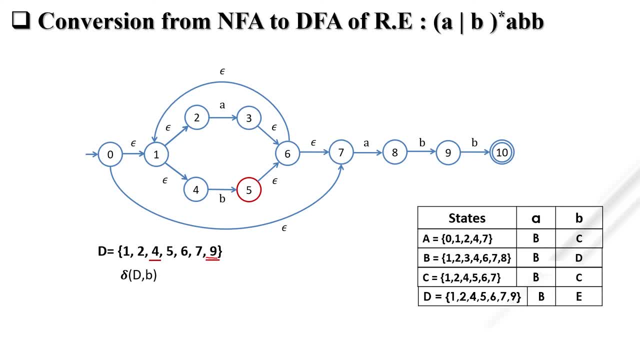 state D. so from 9 there is a transition of B to the final state, that is step. so of B to the final state, that is step. so of B to the final state, that is step. so what is the answer? 5, and so what is the? 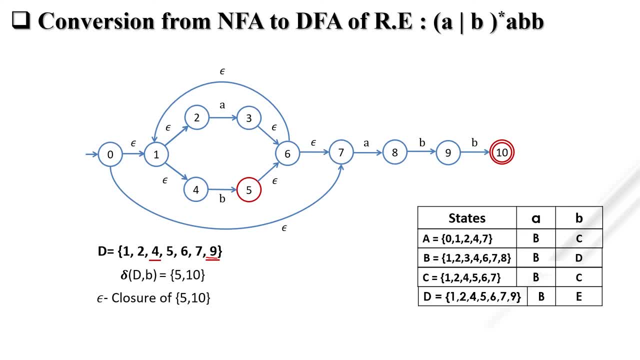 what is the answer: 5 and so what is the? what is the answer: 5 and so what is the null? closer of 5, now, closer of 5 is 5- null. closer of 5, now, closer of 5 is 5- null. closer of 5 now, closer of 5 is 5 itself. then it reaches by taking null to 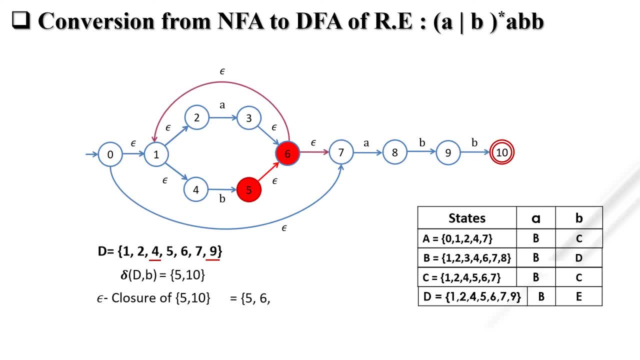 itself. then it reaches by taking null to itself. then it reaches by taking null to 6, from 6, which is 2, 7 and 1, 6 from 6, which is 2, 7 and 1. 6 from 6, which is 2, 7 and 1. from 1, it reaches to 2 and 4. what is the? 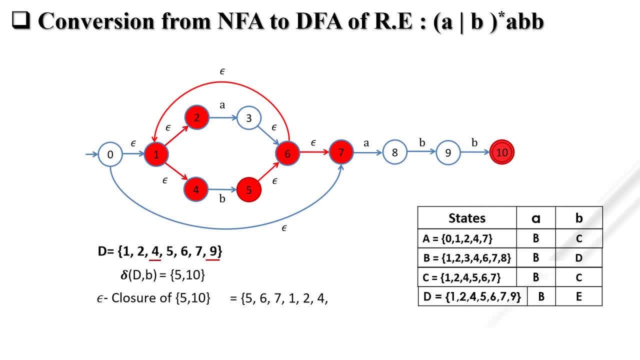 from 1, it reaches to 2 and 4. what is the? from 1, it reaches to 2 and 4. what is the null closer of 10 and itself? because null closer of 10 and itself. because null closer of 10 and itself. because there is no edges leaving out with the. 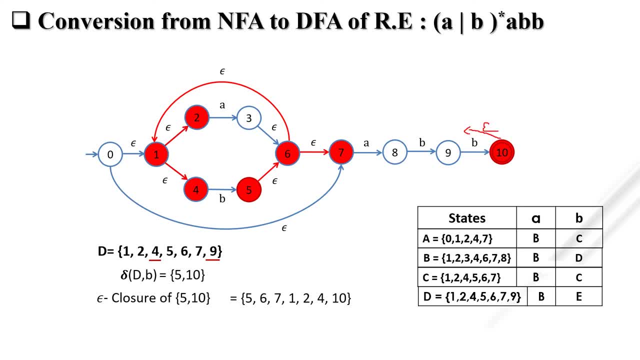 there is no edges leaving out with the. there is no edges leaving out with the symbol now. so this is completely a new symbol now. so this is completely a new symbol now. so this is completely a new state. so we label state, so we label state, so we label this. 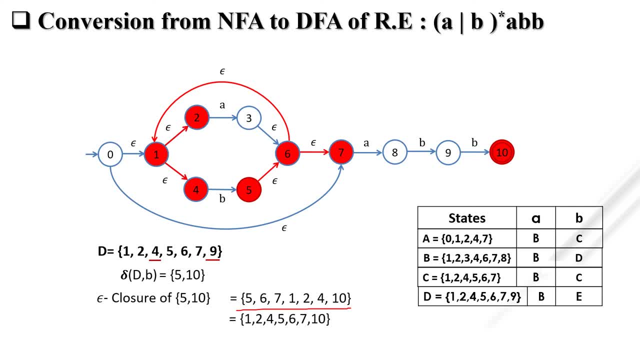 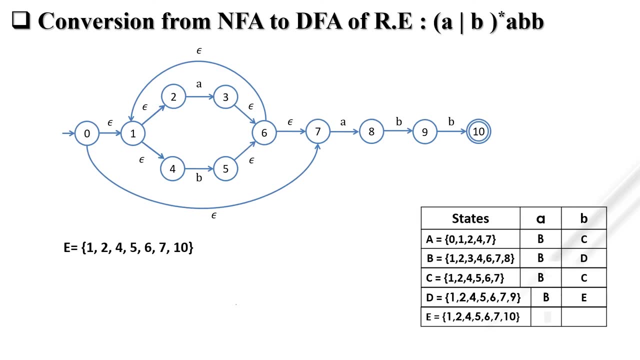 this state as a new symbol, that is e. so we also insert this e in the transition table. now we have to find transition function of e of a and transition function of e of b. so transition function of e of a is what is our e from 1? there is no directly transition. 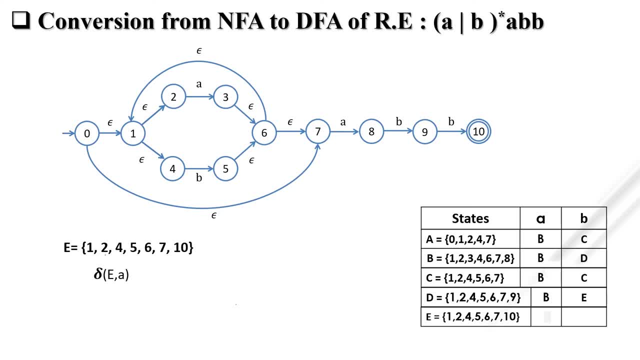 of a. from 2, there is a transition of a to the state 3 from 4. there is no transition from 5. 6 from 7, there is a transition of a to the state 8. from 10, there is no transition of a. so what is our answer? 3 and 8. 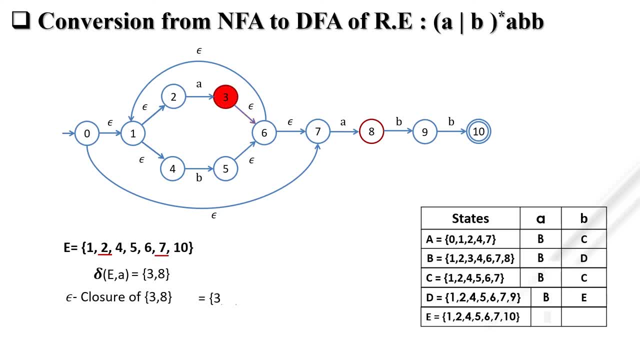 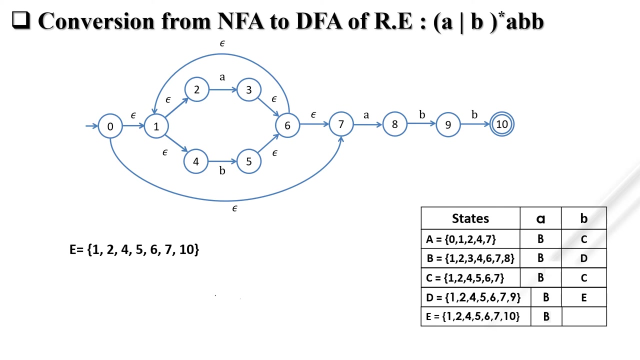 what is null closure of 3 and 8? we already find okay, so we are label this state as a b, because there is no changes in this state, the state b. next we have to find transition function of e of b. so from 1: there is no transition of b. from 2: there is no transition of b. from 4: there is a. 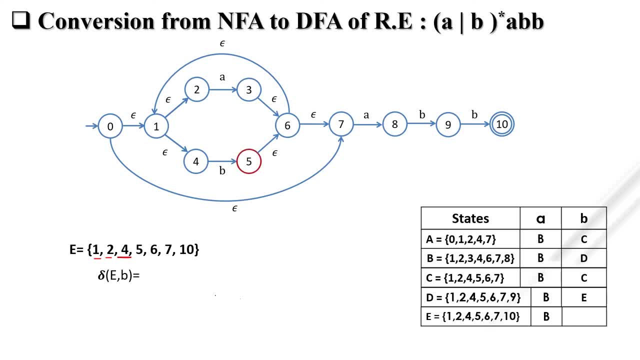 transition of b to 5 from 5. there is no transition of b- 6, 7 and 10. there is no transition of b which reaches to other state. so what is the answer? 5. next we have to find null closure of 5. what is? 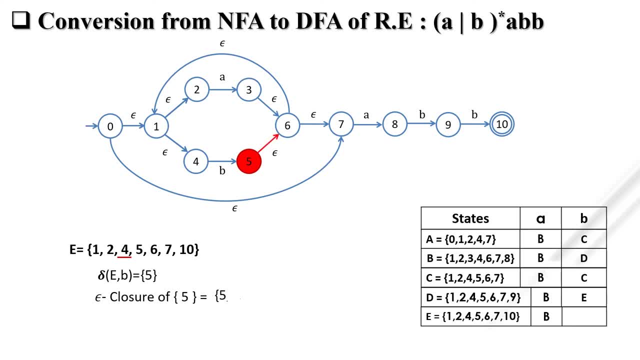 null. closure of 5, 5 itself. and it reaches by taking null to 6 and 7, and 1 and 2 and 4. so what is the answer? 1, 2, 4, 5, 6, 7. so there is no new state because it is already there as a c. 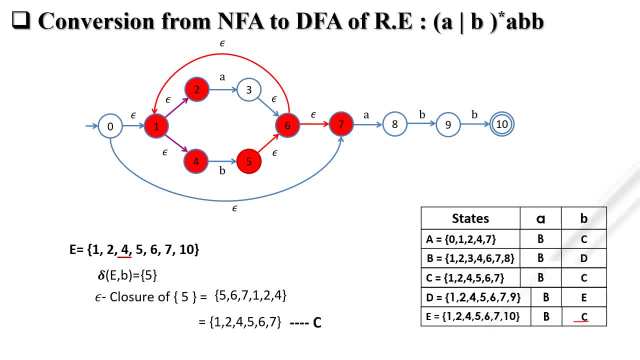 so we label this state as a, c, and what is our answer here? e of b is c, so we complete all the states. so this is our transition table. so we complete all the states. so this is our transition table for dfa. okay, let's see how dfa will be for dfa. okay, let's see how dfa will be. 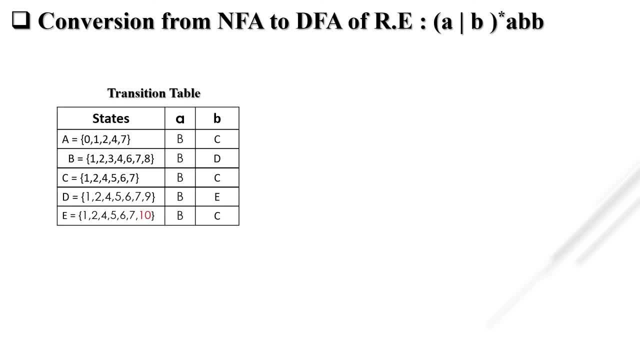 drawn, drawn, drawn, drawn. so this is a transition table for DFA. we get this table with the help of subset construction method. okay, so let's see how we draw the DFA with the help of this table. so what is our initial state as we first find the null closure of 0. 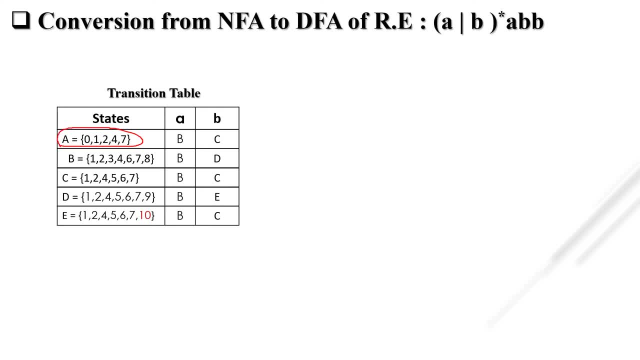 and we get this a. so a is our initial state. so what is our transition function of A of A? we get the new state that is B. so we simply draw a edge with the symbol A, which reaches to B. similarly, what is our A of B? we reaches to C. so 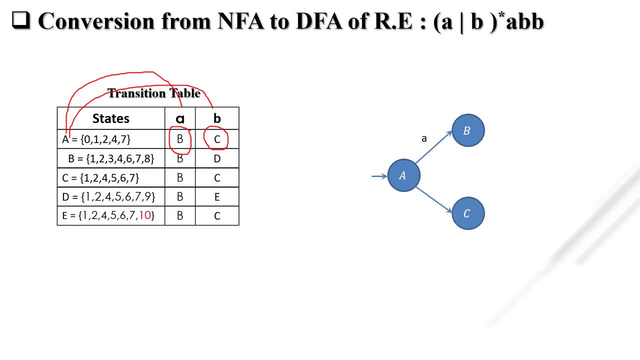 from A, there is a new edge which reaches to C with the symbol B. so, similarly, from B of A, there is a self loop. okay, so we simply put a self loop with the symbol A. from B of B, what we get, we get D. that is a new state, so we draw one new. 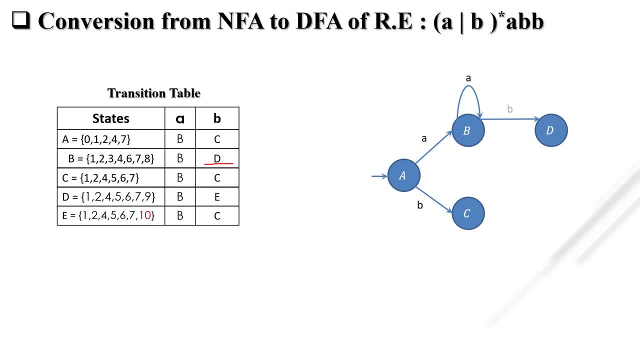 state and pass one edge with the symbol B. now, what is C of A? C of A is B. so what we do? we pass one edge from C to B with the symbol A. similarly, what is C of B? we get C. that is self loop with symbol B. 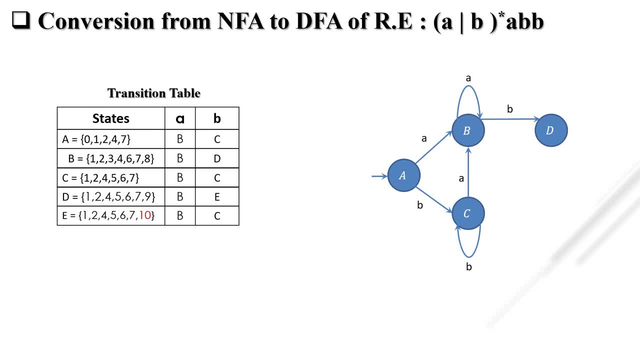 what is our D of A? D of A is B from D. there is an edge with the symbol A reaches to capital B. what is our D of B? it reaches to capital E. so we have to form one new state, that is E, with the symbol B. similarly, E of A: it reaches to capital B. 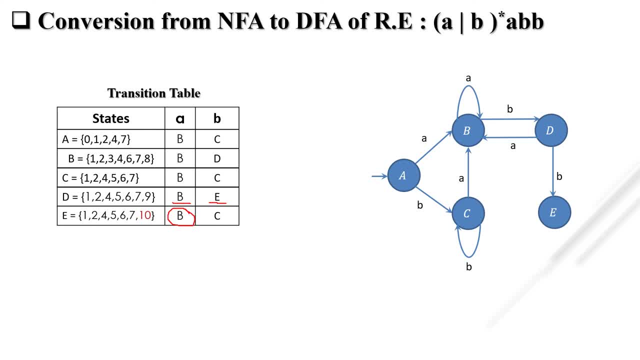 so we pass one edge from D to B with the symbol C. similarly, from E to D, we pass one edge with the symbol B. okay, so what we have is D of A. this is our D of A. what is our accepting state? this is our accepting set. 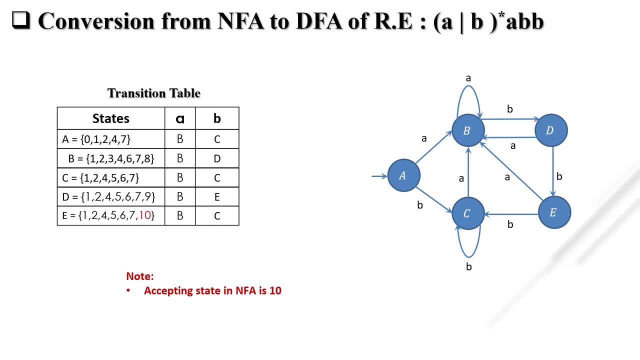 Accepting state of NFA is 10. okay, when we draw an NFA, the accept state is 10. so now we check in which of the state this 10 will be there. in A, there is no 10. in B, there is no 10. in C, no. in D: no in E, there is a state 10. so 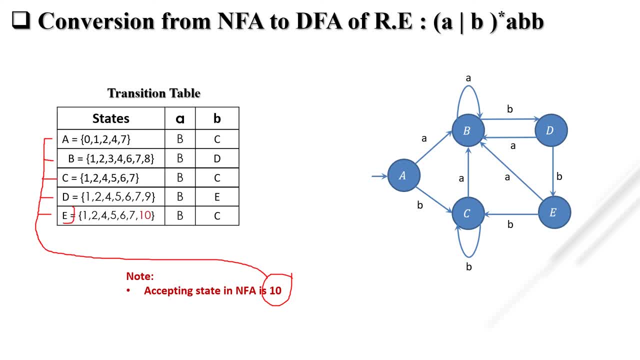 we considered this E as a final state. now it may be possible there is more than one final state. okay, so don't be confused. in another example it may be possible there is two final state or three final state. what is our final state E? so this is our DFA for the re a or B, the whole star, a, BB. so you can clearly see. 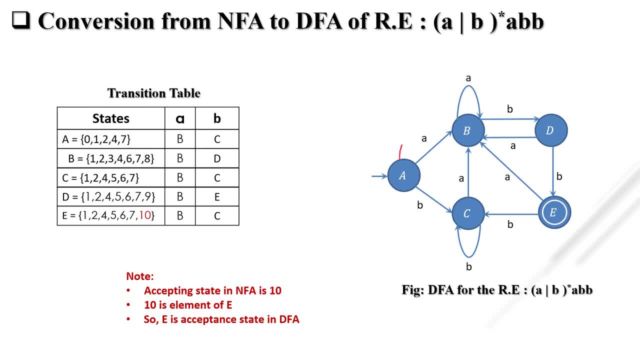 that from a, there is a only one edges living out with the symbol a. there is no other edges living out with the symbol a to another state, okay. similarly, from B, there is a symbol B which is living out to D, but there is no other symbol, no other edge with the. 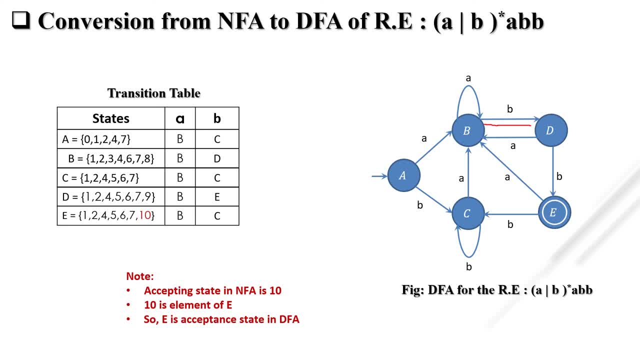 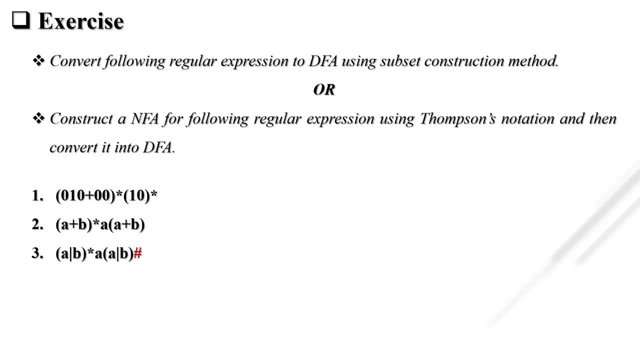 symbol B which reaches to another state. so this is our correct DFA. so this is exercise that you have to do by yourself. the question may ask in two ways, like: first convert the following regular expression to DFA using subset construction method or construct NFA for the following regular expression using: Thompson notation and then convert it into ste comptroller. again, I'm still not. so we have to convert this DFA with the help of subset construction method. now if such a flying is given, all the say he does notice like a say. I am very diligent, often like I walk 10 to. expert should fail. sometimes you can. 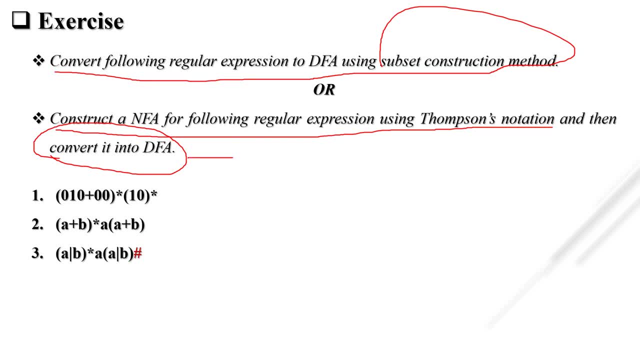 I effort to try and reverse fall. so what we did is that everything again this circle summer around, we all, we will focus in. okay, also, this has symbol is a end marker, so don't be confused. this is end marker. you have to consider only this string to draw the dfa. okay. 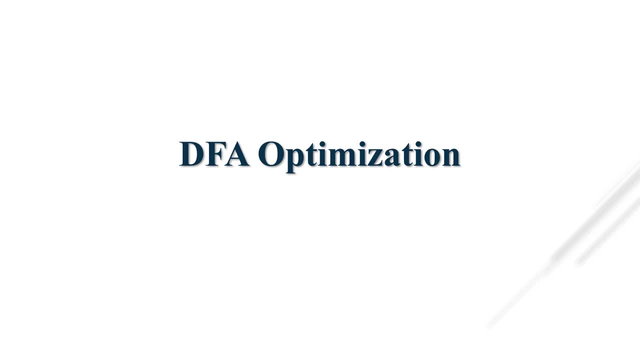 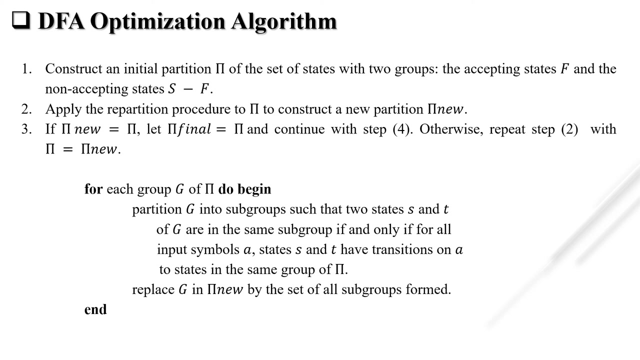 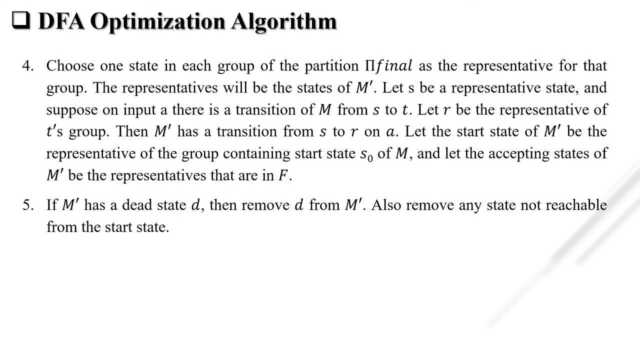 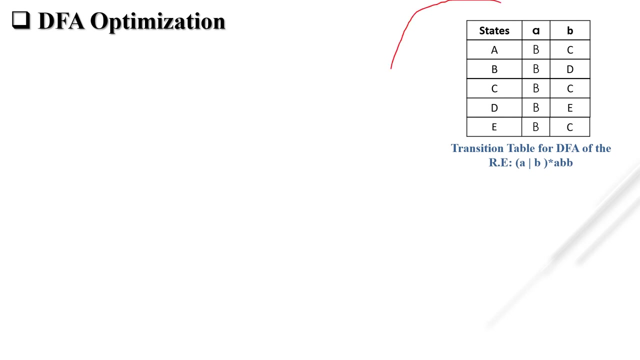 so the next topic is dfa optimization: how we optimize the dfa with the help of transition table. so this is an algorithm for dfa optimization. let's optimize first and then you see this algorithm. you clearly understand, okay. so this is a transition table of dfa that we already discussed earlier for 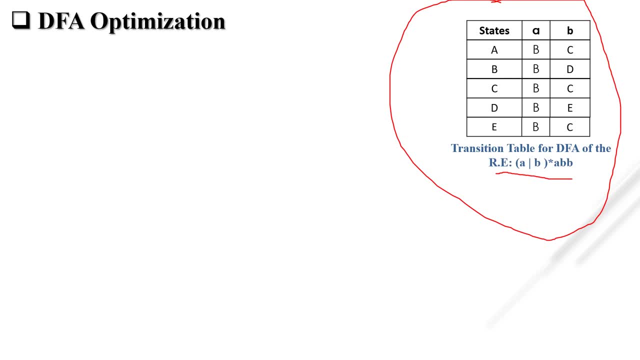 the re a or b, the whole star a, b, b. let's see how this dfa will minimize. so there are total five states, that is, a, b, c, d and e. so first we separate the final non accepting state and accepting state. so what is our accepting? 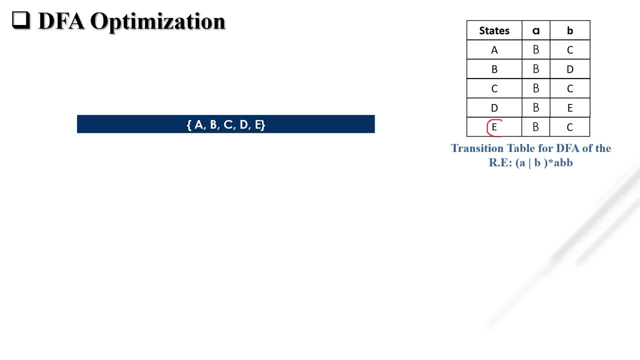 state in that dfa, e is our accept accepting state and a, b, c and d are non accepting state. so we split first these two in two different state, so in zero equivalence we get two: a, b, c, d in one part and e in other part. okay, 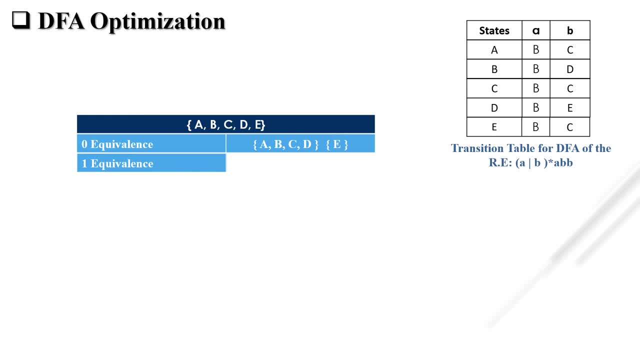 so next one is: one equivalence in one equivalence. what we do, we check a with b, that a and b are equivalent or not. for that, what we do, a of a and a of b are going to b- okay, it is already in this set- and a of b. 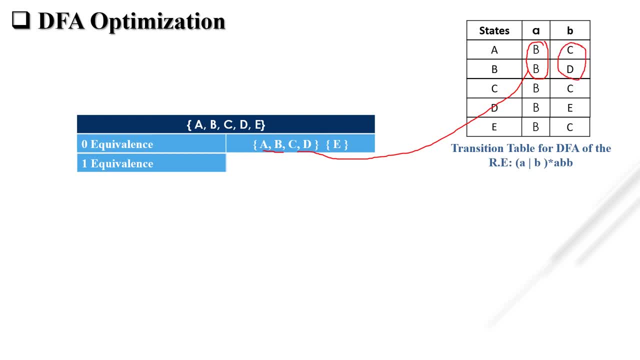 and b of b is going to c and d. this all are also in this set, so they are one, equivalent to each other. that is a and b. now we check a and c or b and c. okay, you can check with a, you can check with b, because a and b are both one. 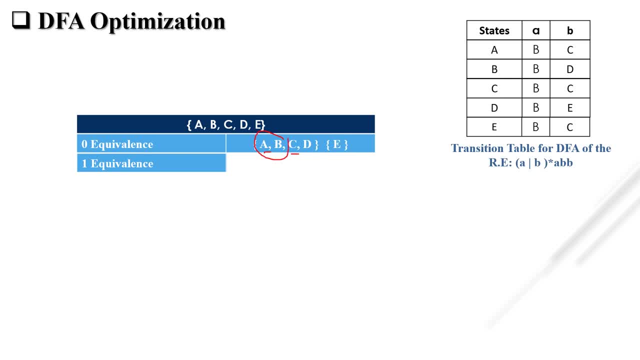 equivalents. so let's check a with c: a of a is going to be, c of a is going to be. okay, this is under this set of already, so c of b is going to c and c of c is going to c. this both are also in this set, so they are also one equivalence to each other. 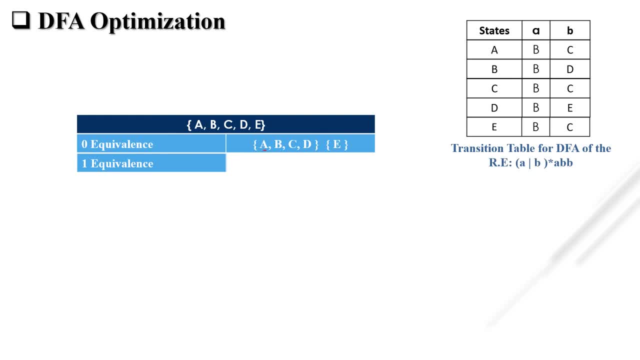 now we check a and d. you can check b with d, c with d or a with d. okay, because a, b, c are one equivalence to each other. so i will check with a. so a of a is b and d of b is sorry, d of a is b. 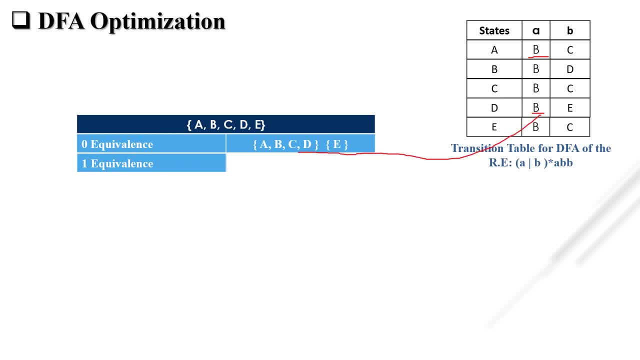 both are in the set. yes, now, a of b is c and d of b is e. so c and e, both are not in this set. so we split d. okay, we separate d. so by separating d in one equivalence, what we get? we get a, b, c, d and e. 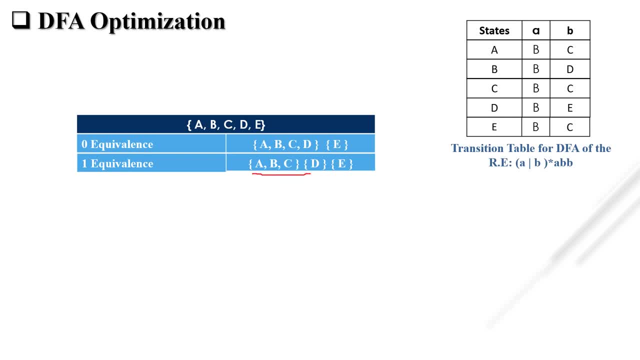 so now we check this for two equivalents. okay, we are not checking this one, not checking this one. now we have checked this first equivalence to get two equivalents. so we check. similarly, we check a with b. what is a of a and b of a- b? both are in the set. 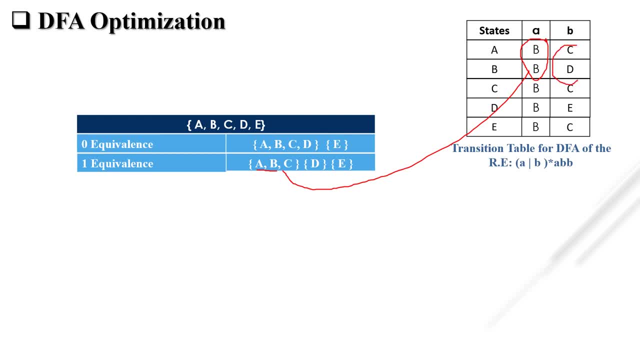 now, what is a of b and b of b, c and d? okay, so we, as d is not in this set, so we separate this b. okay, now we have to check this c. c goes where in the set a or in the set b, for that first we check. 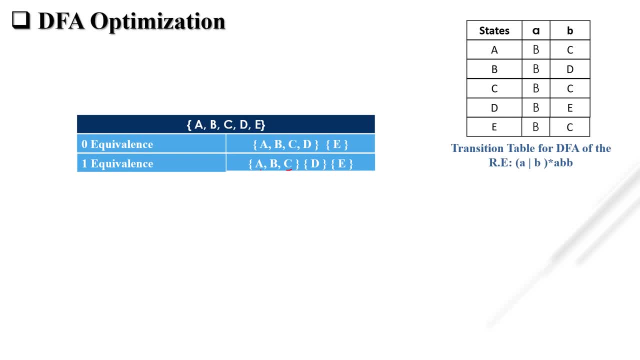 c with a, okay, c with. what is a of a? it is b. what is c of b? sorry, c of a, it is b. both are in the same set. okay, they are equivalents. now we check a of b, a of b, what we get c, what is c of b, what we get c. both are in this set, okay, so a and c. both are remaining together and we will separate in two equivalents. 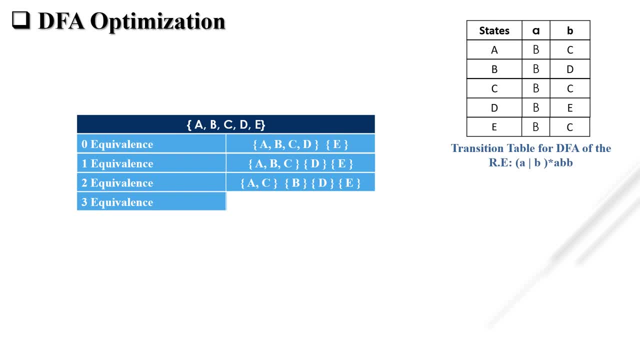 now in third equivalence we have to check a and c only because b and d and e are already separated, okay. so what is a of a? a of a is going to be, c of a is also going to be okay. so there is no problem. now we check: a of b, it is going to c, and c of b, it is also going to c. 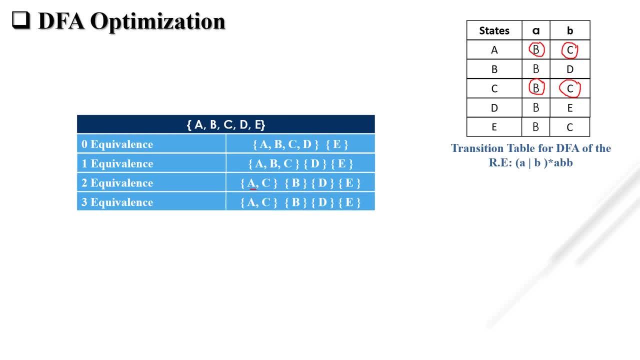 so a and c is not going to separate. so in two equivalents and three equivalents, the answer remains same. so we are not going to four equivalents. we stop here. okay, so there are no more splitting is possible. so if we choose a as a representative for the group a and c, 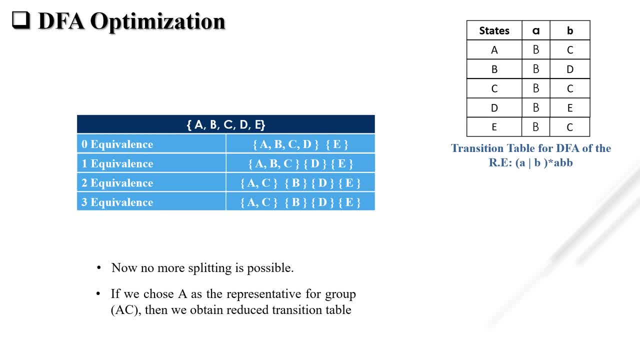 then we obtain the reduced transition table. okay, so instead of a and c, we write differently. we represent this c as a. okay, so we delete this row. so what we get, we get a and c. a of a, b and instead of a of b is going to c. 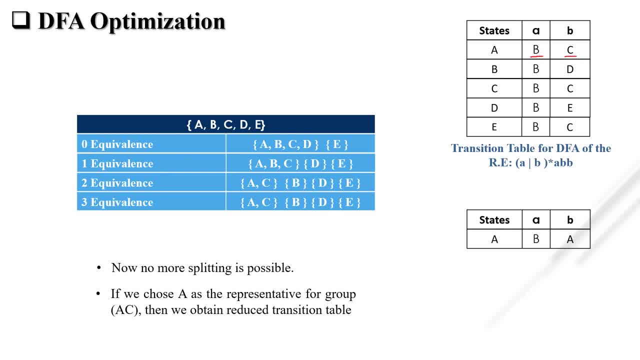 what we write. a, because the representative of a and c is this: a. next b is going to b, b of b is going to d. now this one is deleted. what is d? d of a is going to b, d of b is going to e, e of b is going to sorry, e of a is going to b and e of b is going to. 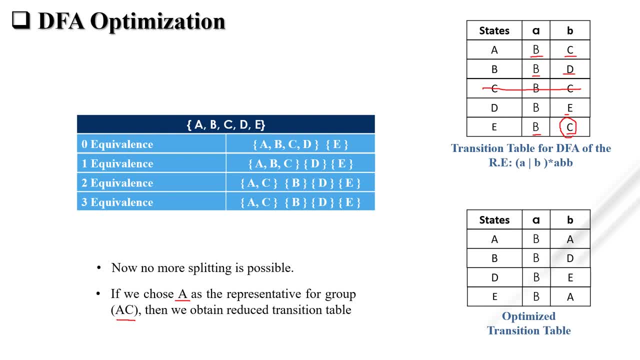 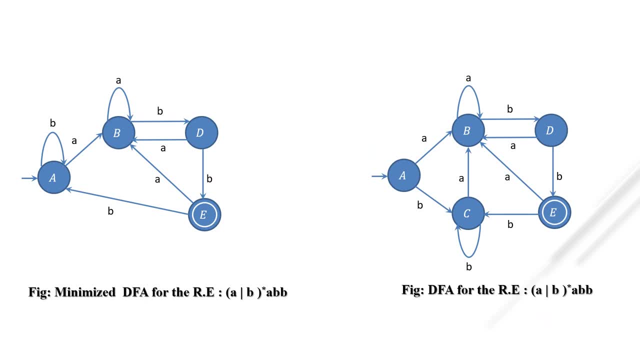 a instead of c what we write a. so here you see, in dfa we have total five states: a, b, c, d and e, but in minimized dfa we have only four states. so you clearly see that this is a class b and we should only nutrients to theЖn.